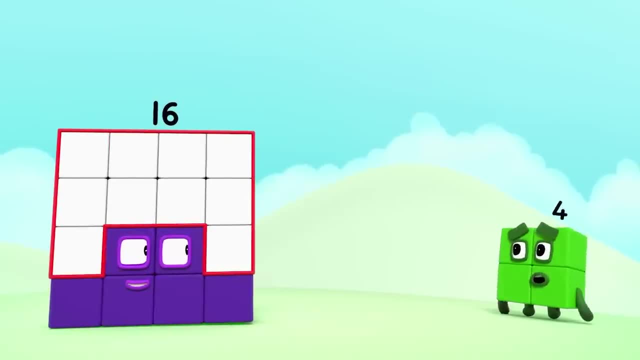 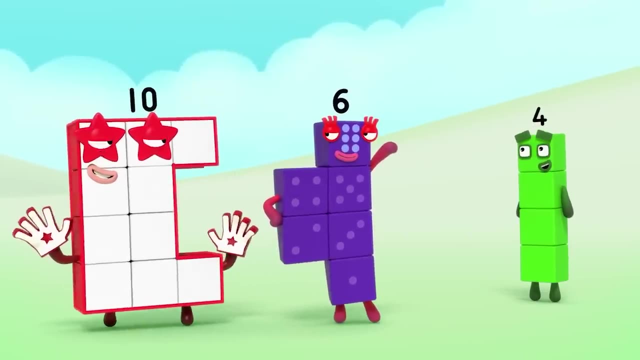 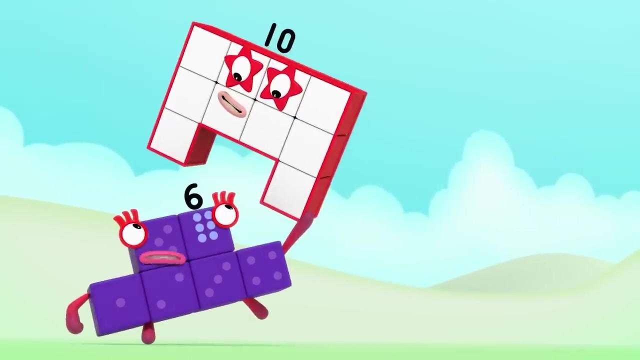 But I've got 16 blocks Square, Really big square- 16. 10 and 6.. I like this game. 16. 10 and 6. Party 16. I am 16. I'm 10 and 6.. 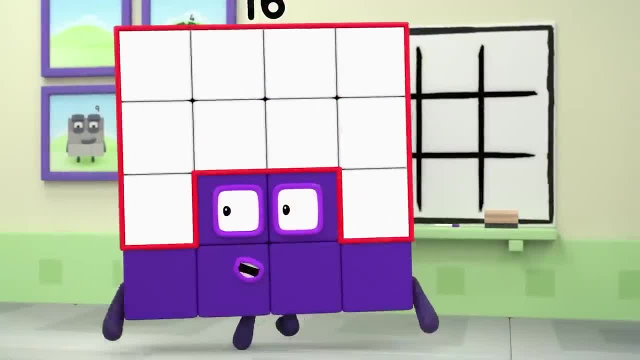 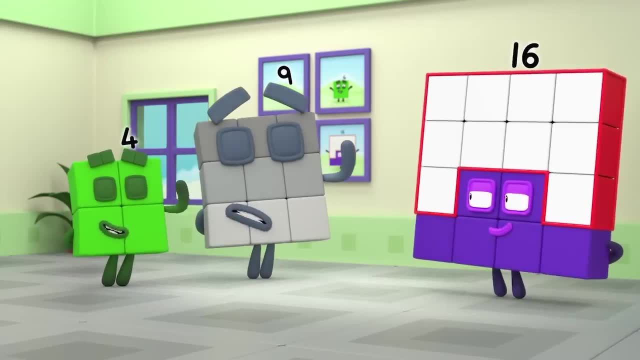 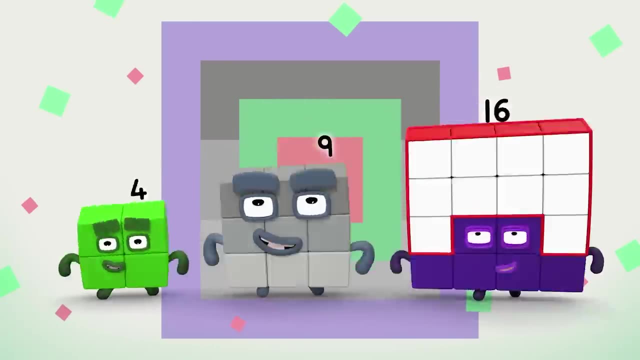 And I've got loads of party tricks. Now we're all here and square, we can begin. What's the first rule of Square Club? No, round things. Right, you are. And let me hear the motto: Even though we're different sizes, you can always recognise us. 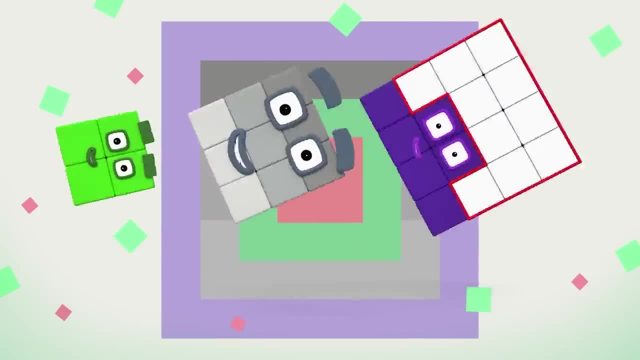 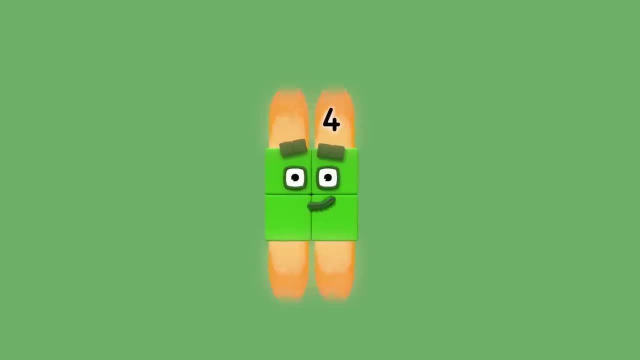 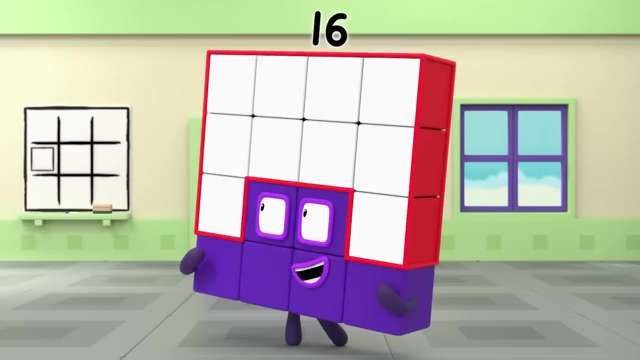 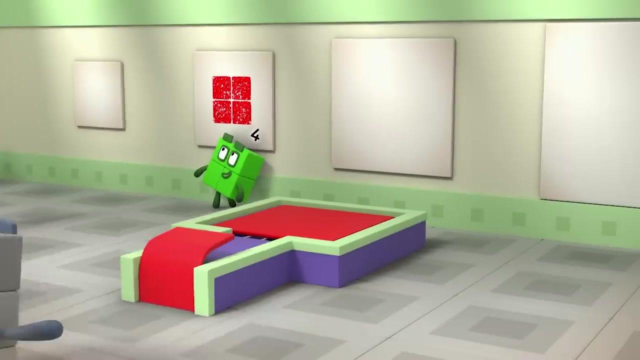 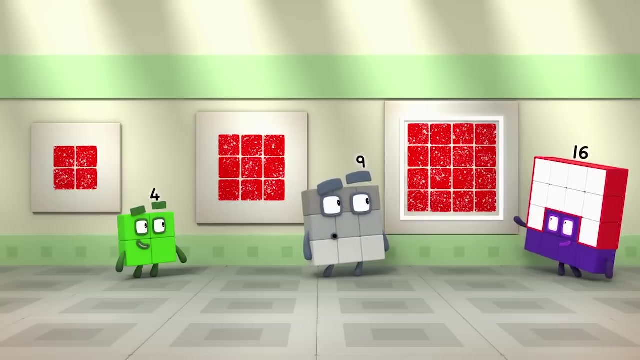 We're as tall as we are wide. We're the same tall on each side, 4 by 4.. 3 by 3.. 2 by 2.. Square Club Hooray: Time for some square art. My square has four sides all the same and four corners all the same. 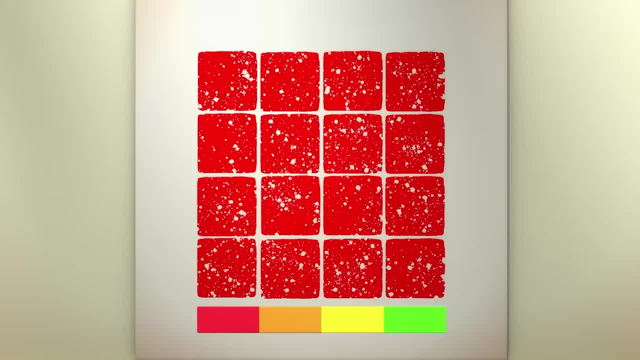 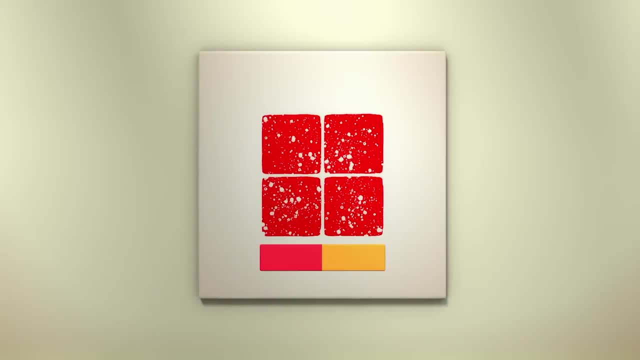 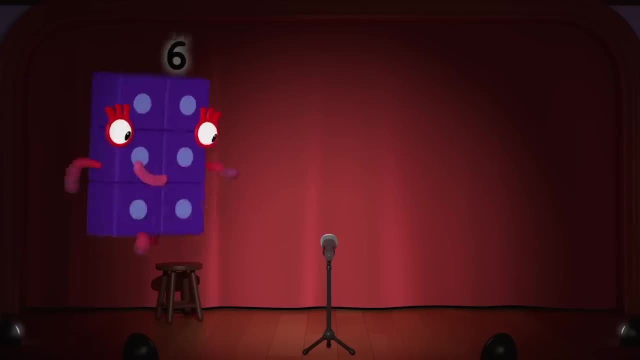 So does mine. Mine too. Mine's four across by four down, Mine's three across by three down, Mine's two across by two down. Let's do something good. I just want all of you to know that it doesn'tmoments happen directly. 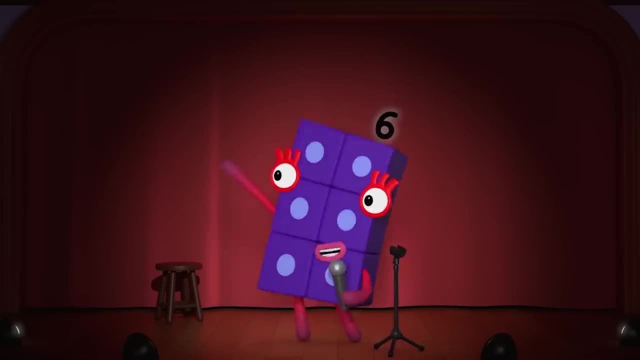 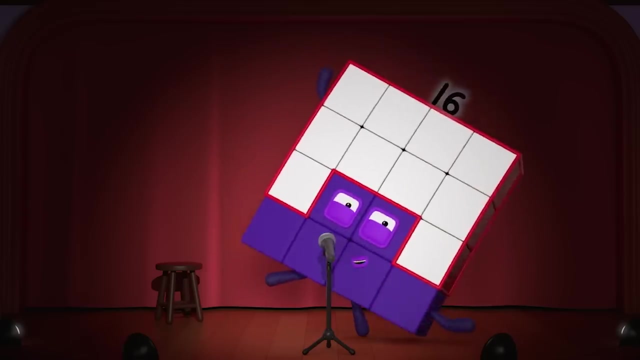 Well, all you'll do is fire with all the lights required and sit, Go on. No, don't look, That's ten guys過去 into a ten. Welcome to 64. Chapter 16.. A six walks into a ten. 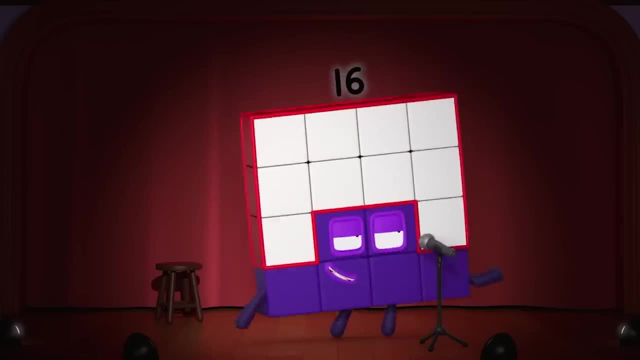 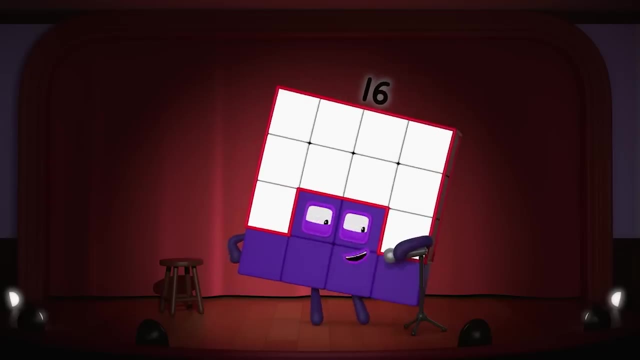 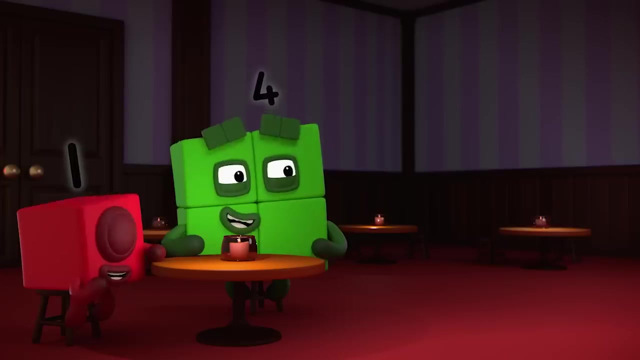 And here and here and here. Oh, look at that, I'm a square turning round. Hey, you know what nine's favourite story is? Goldilocks and the three squares Squares. And if you're after a square deal. 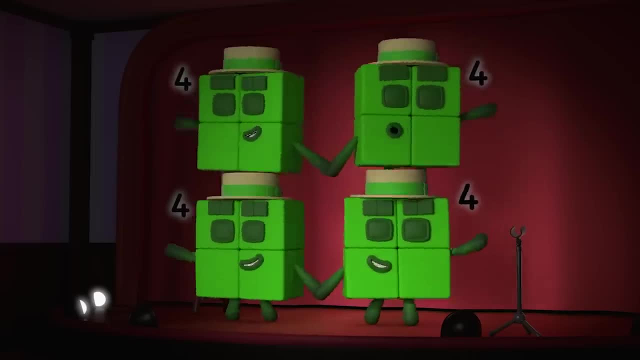 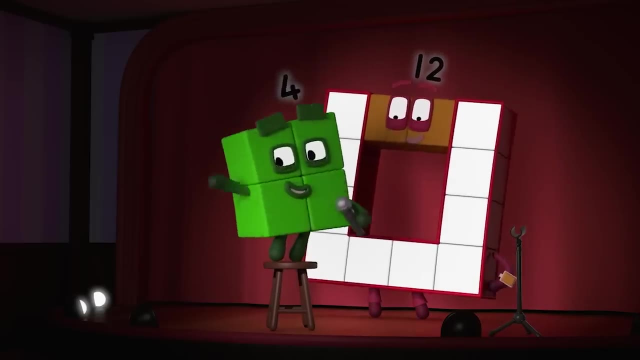 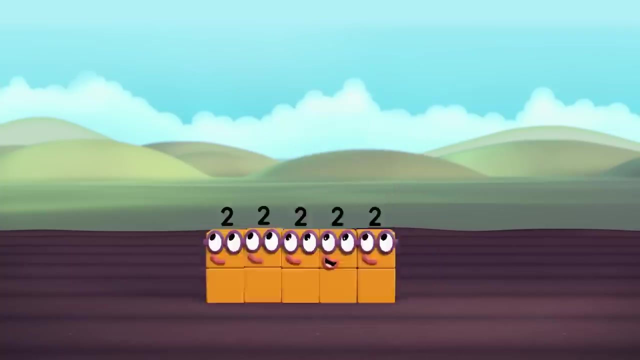 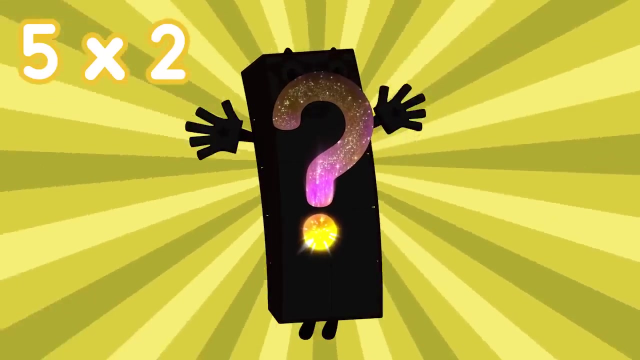 here I am. I'm a square Made of squares, With a A square In the middle. So much faster. Ten, go again On your marks. There are five of us. Five times two equals Ten. I am ten. 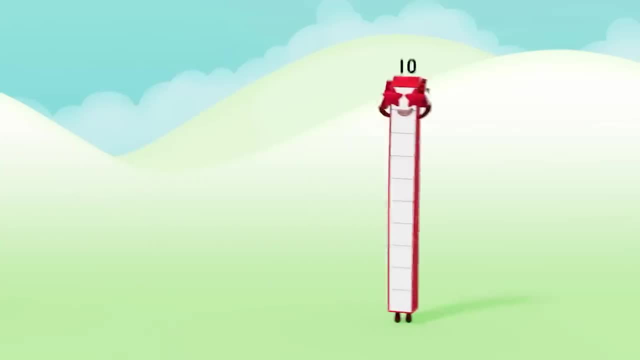 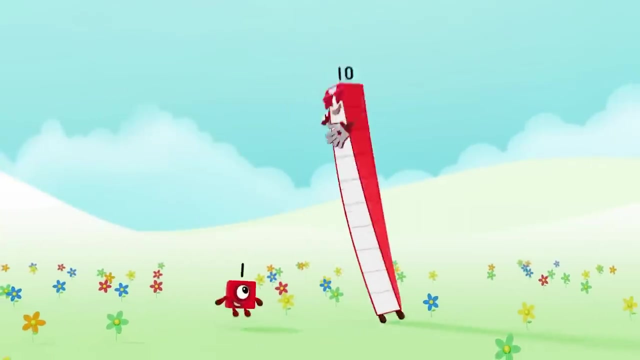 Watch this: Ten Minus one equals Nine. Nine, Ten- You're amazing. One bigger. You're one bigger. Why do you have a one on top? If you're wondering why there's a one on top, you'll know the answer when you realise. 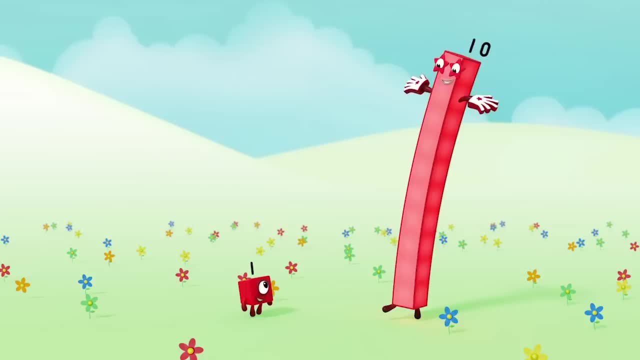 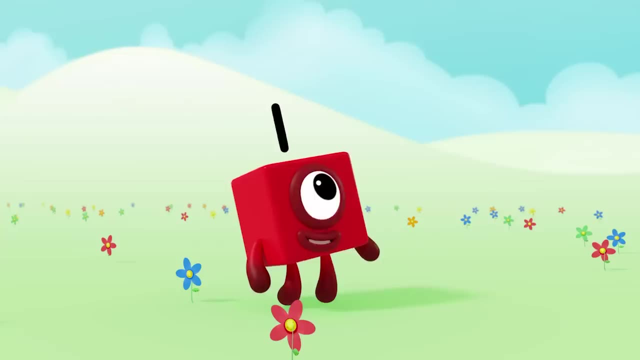 I'm one big block. I'm one big, perfect ten. I'm a ten block. I'm a ten block. You might think we're. We're more alike than you suppose. You're 1-1 and I'm 10-1's, which means 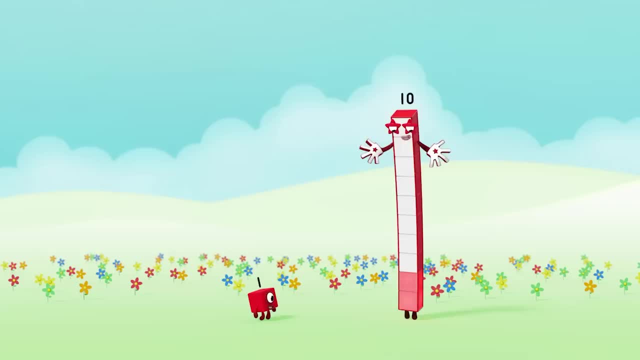 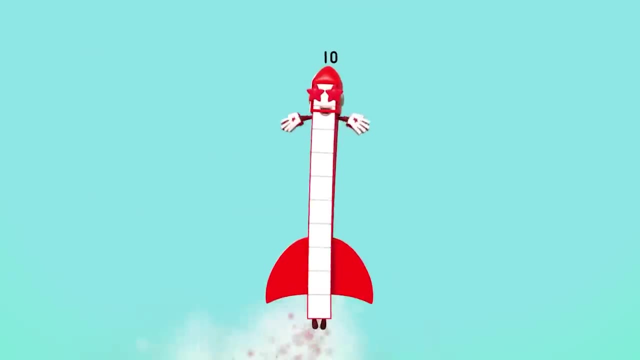 I'm 1-10: 1,, 2,, 3,, 4,, 5,, 6,, 7,, 8,, 9,, 10, I'm 10,, 10,, 10, And I'm flying through the sky. 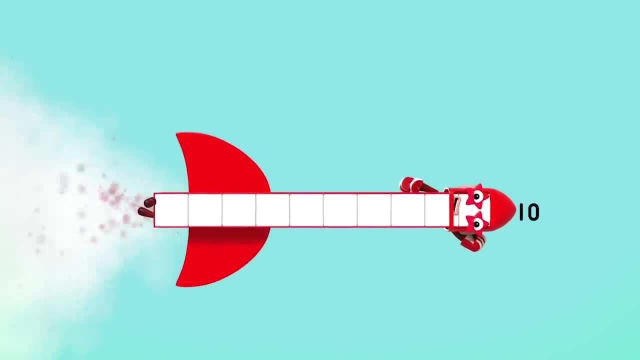 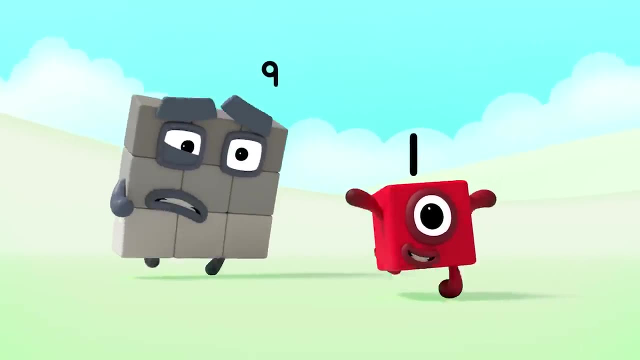 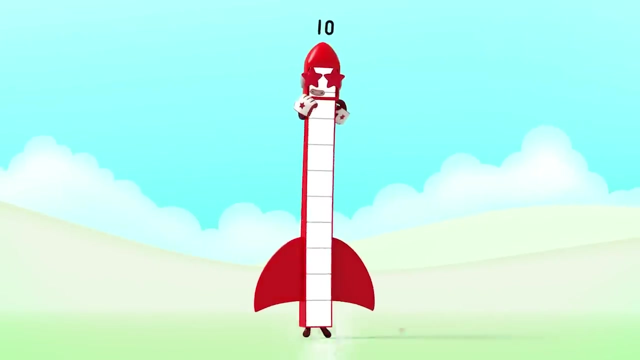 I'm 10,, 10,, 10. You can break me up any way you like. I can be 9 plus 1, going for a run, Trying not to sneeze And having lots of fun. And then I'm 10,, 10,, 10 again. 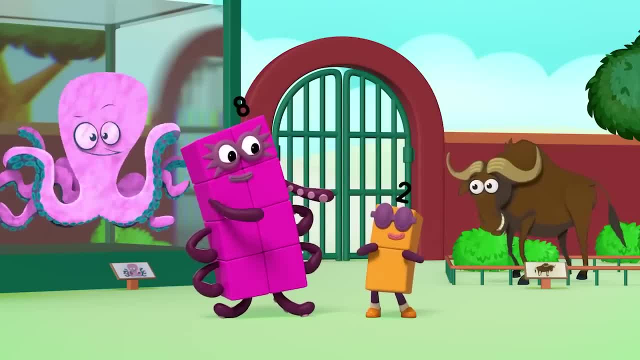 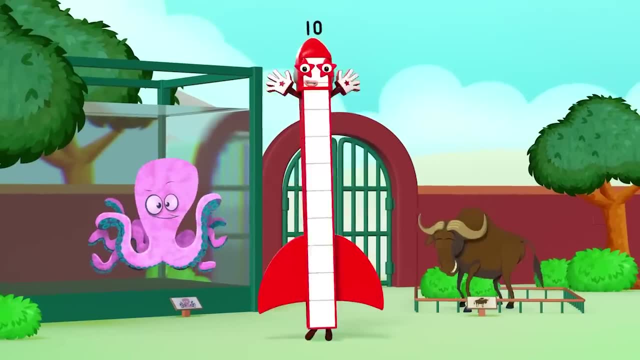 I can be 8 plus 2, visiting the zoo, Talking to the octopus And dancing with a canoe, And then I'm 10,, 10,, 10 again. I can be 7 plus 3, 7 plus 4,, 3,, 2 and 2. 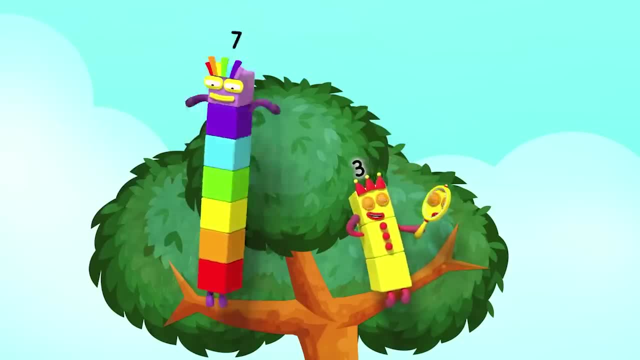 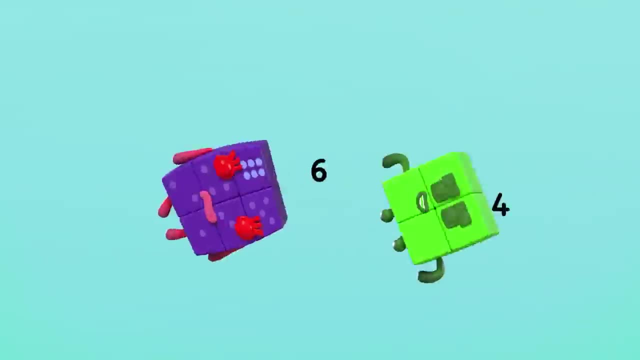 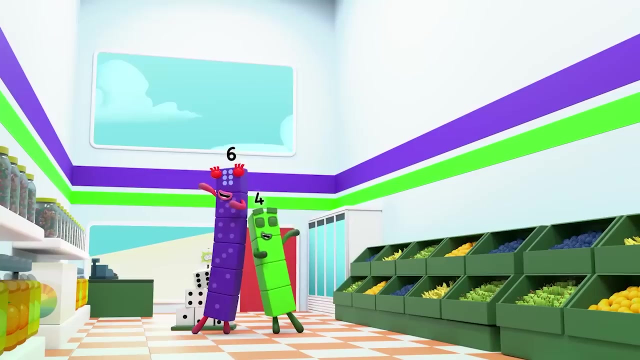 7 plus 3,, 2 and 2 Sitting in a tree making rainbows, but looking at me, and then I'm ten, ten, ten again I can be. six plus four. shopping at the store playing with a dice on a square tile floor, and then I'm ten, ten, ten again I can be. 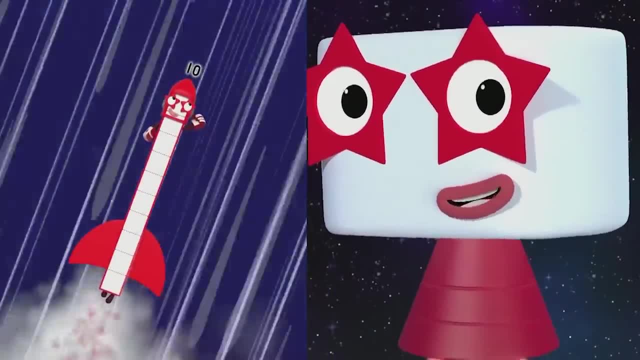 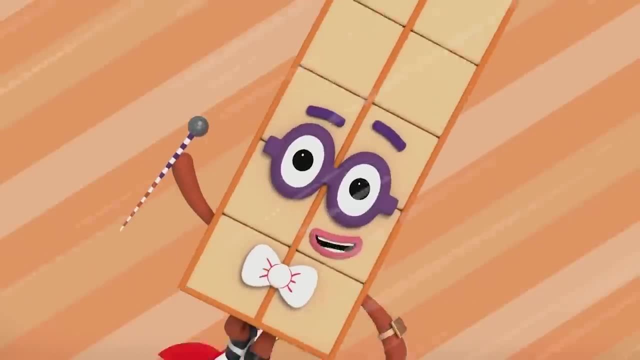 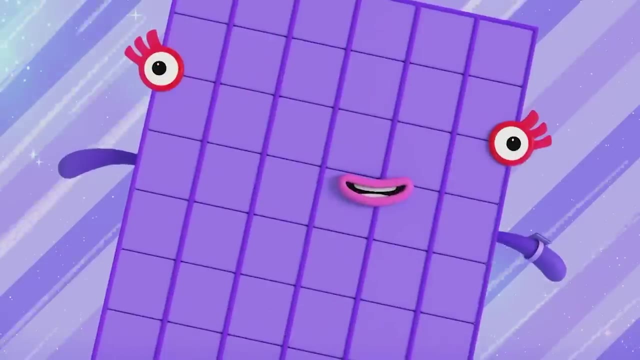 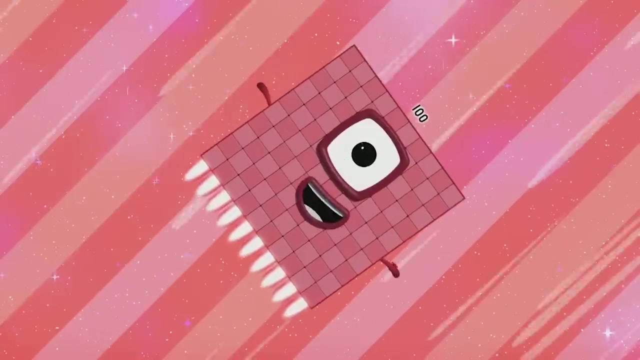 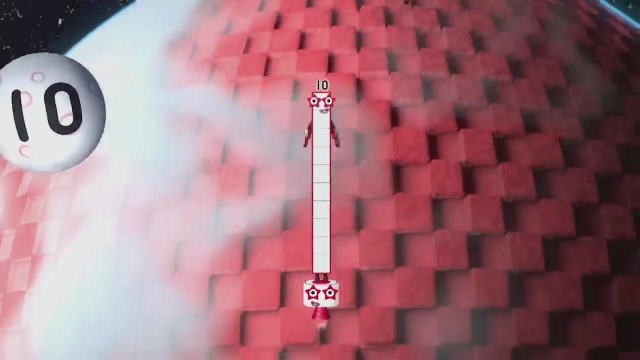 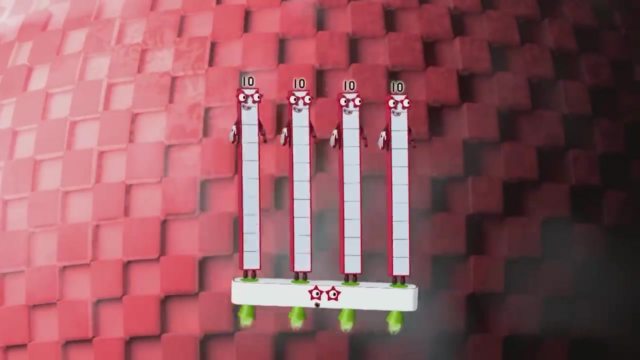 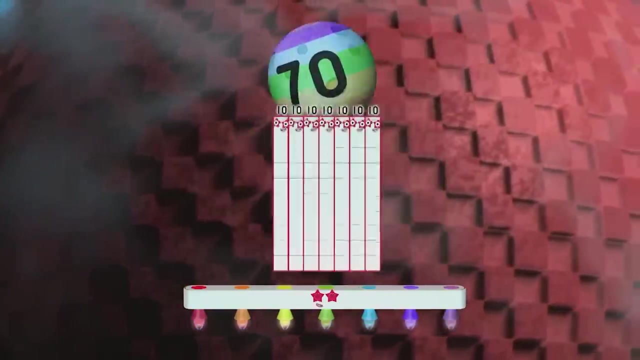 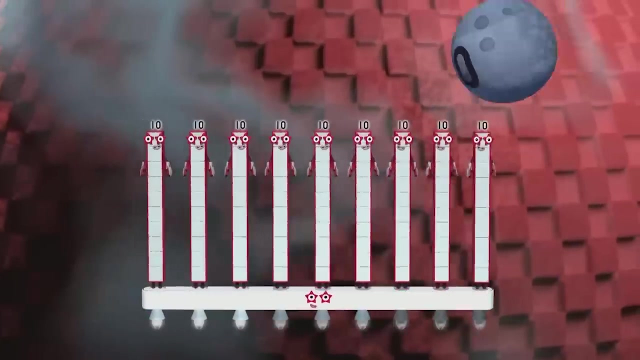 Heroes with zeroes. this is the ten times. table rocket rescuers. come as soon as you are able. ten, twenty, thirty, forty, fifty, sixty, seventy, eighty, ninety, one hundred heroes with zeroes. one ten is ten. two tens are twenty, three. tens are thirty four. tens are forty. heroes with zeroes: heroes with zeroes. five tens are fifty six. tens are sixty, seven. tens are seventy, eight. tens are eighty. heroes with zeroes: heroes with zeroes. nine tens are ninety and ten tens are one hundred. heroes with zeroes. heroes with zeroes. 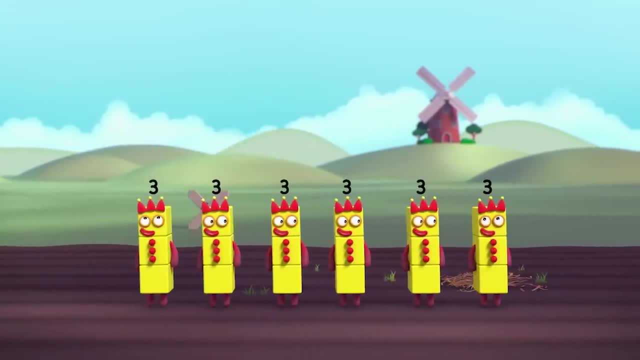 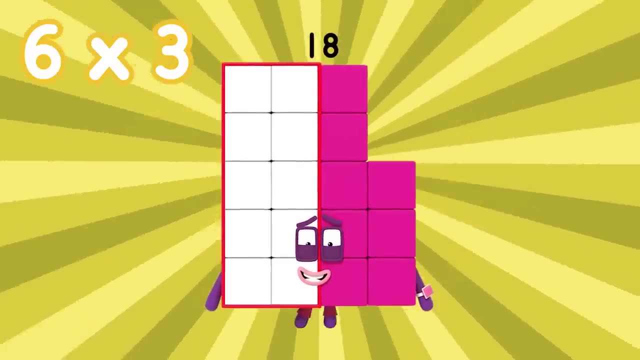 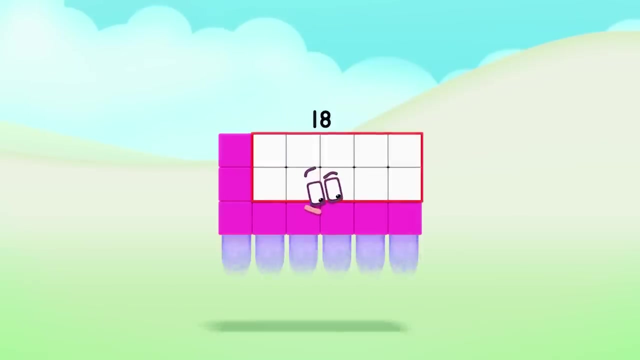 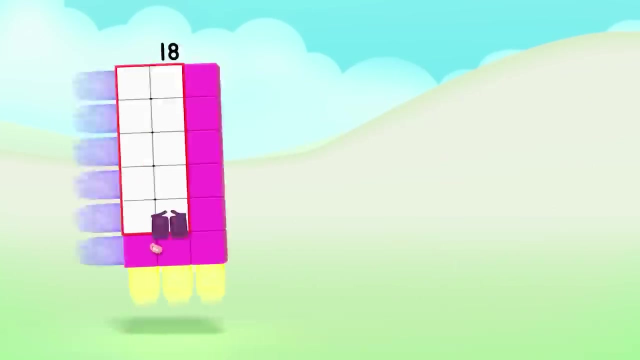 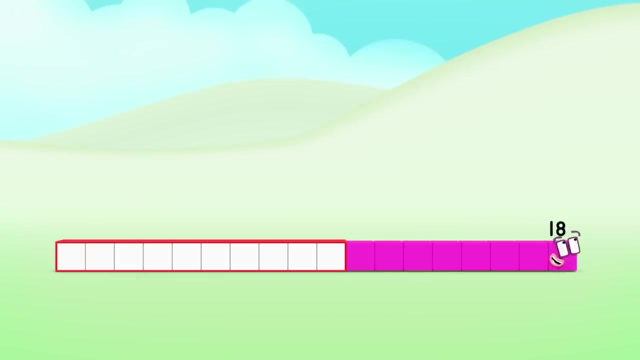 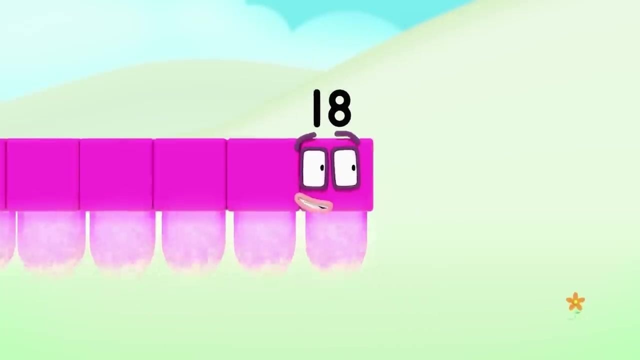 I turn. six times three equals eighteen. hey time to discover who I am done. I am eighteen and I'm a super speedy, super rectangle and I like to go fast. so tall ooh, falling over competition, ah oof. I win, ah-ha, eighteen by one. one ray is all. I need one ray to build up speed. I start to go and I go, go, go, whoa ha-ha. 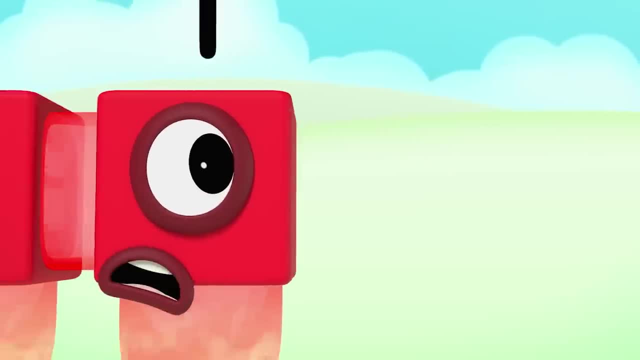 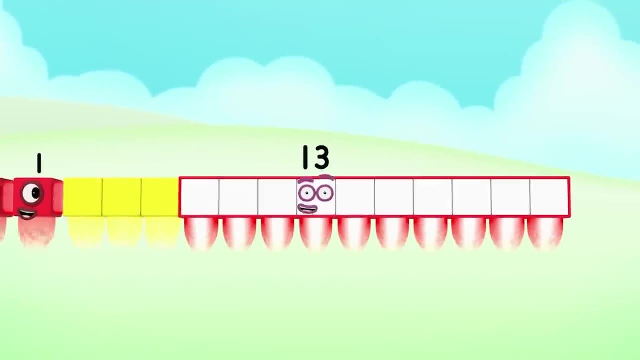 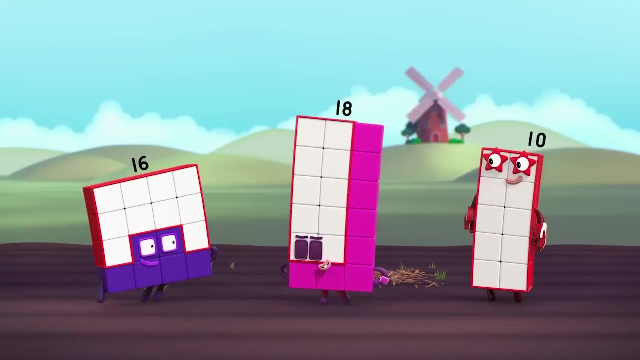 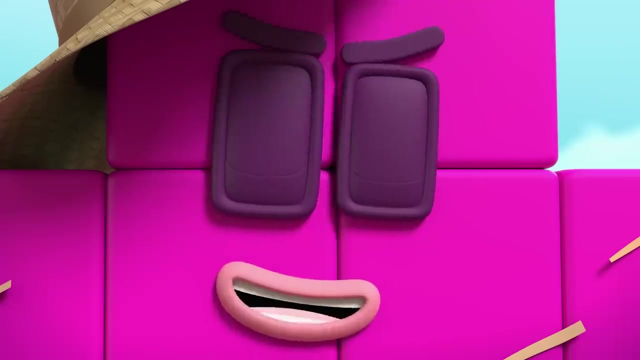 eighteen ones. this is fun too fast. one, two, three, four, five, six, seven, eight, nine, ten, eleven, twelve, thirteen, fourteen, fifteen, sixteen, seventeen, eighteen, ha-ha ha, refreshingly fast. this makes up for breaking some silly old scarecrow. whoops, eighteen, eighteen, no, I can't see any eighteen, just this good old scarecrow. 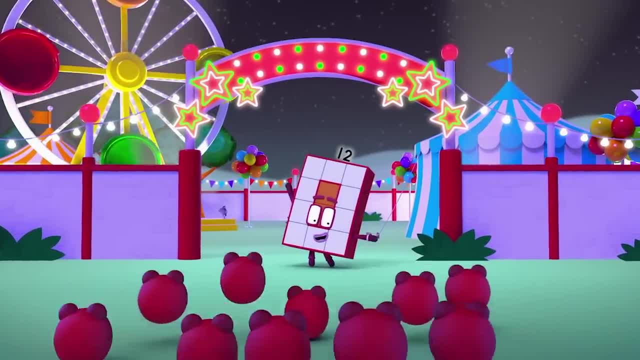 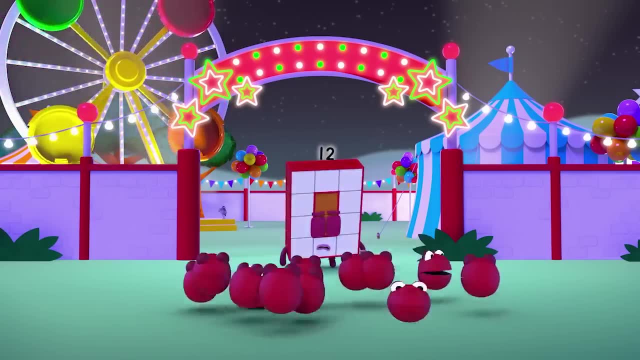 ooh, how interesting. I can't believe I'm riding a horse. ooh, I'm riding a horse. ooh, I'm riding a horse, ooh, ha-ha. welcome to the fun times. back is everyone here. one, two, three, one, two. oh, come here. 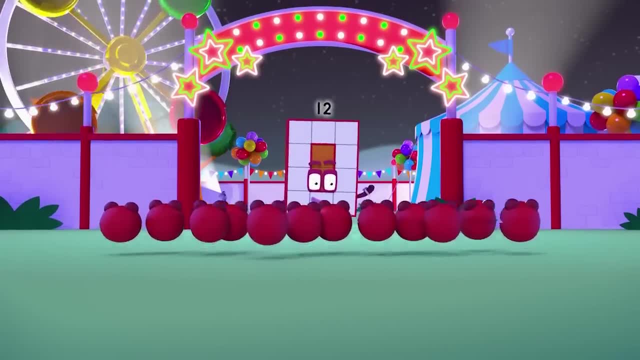 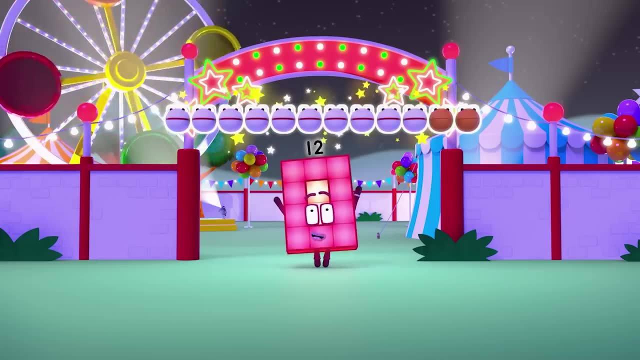 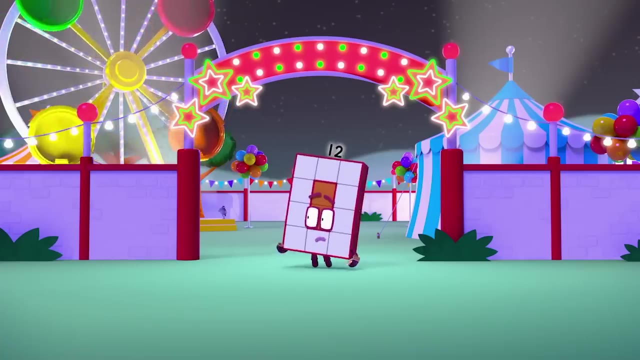 ooh, one, two, three, four, five, six, seven, eight, nine, ten, eleven, twelve, twelve, number blobs. good, I've got lots of ride tokens. what would you like to? thirteen The teacups, The teacups. 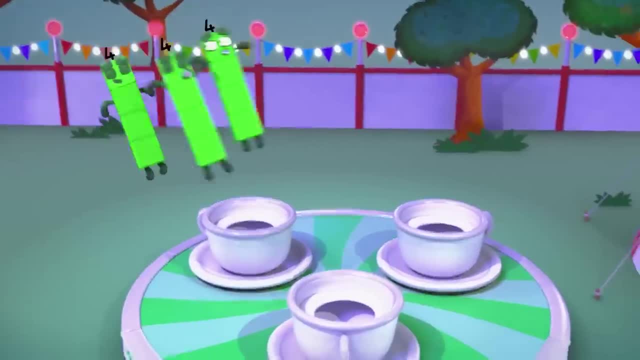 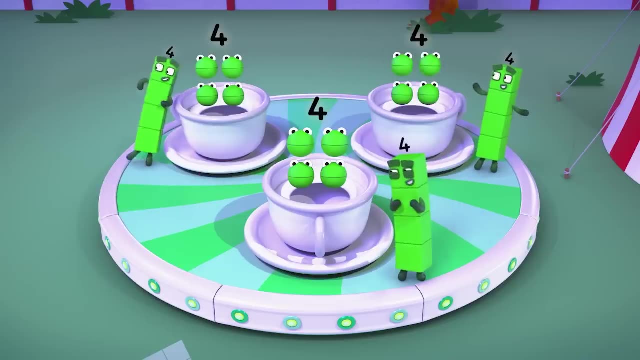 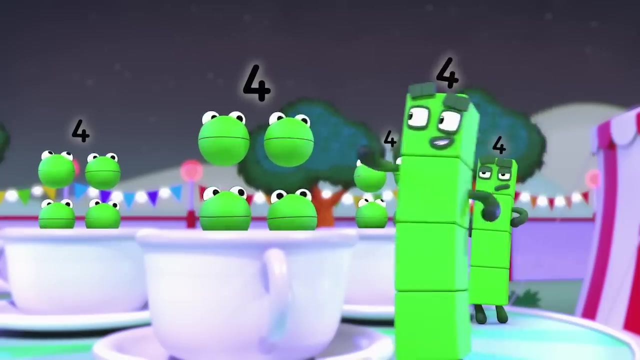 It looks like four to a cup. One, two, three, four. One two, three, four. One two, three, four. Now, how many ride tokens do you need? Um, Look at it this way: How many cups are there? 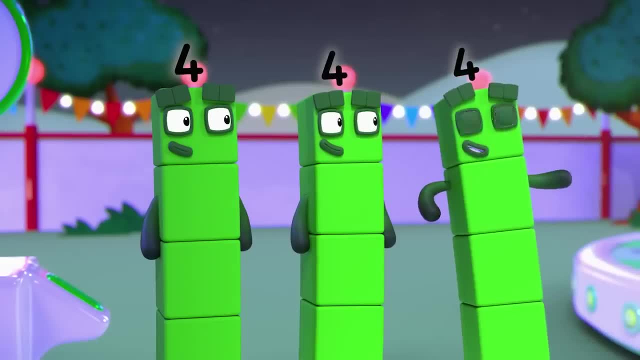 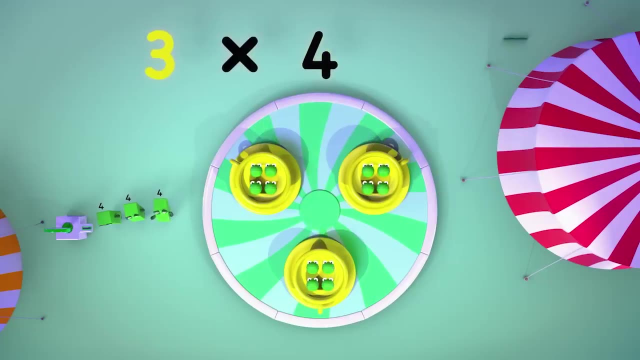 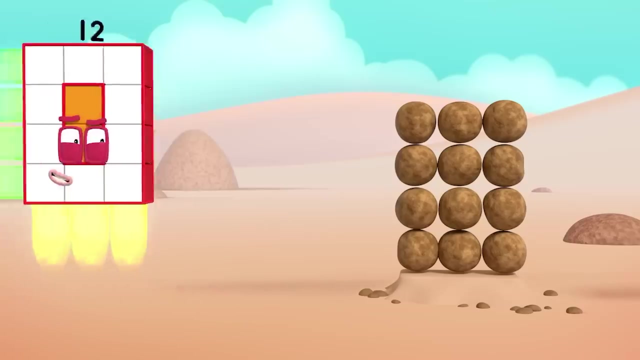 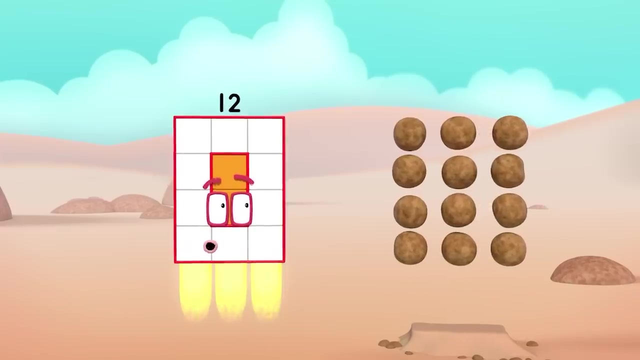 One, two, three, Three cups And how many riders in each cup? Four. So that's three. lots of four, Three times four, which is Twelve. The rocks are in columns and rows. My blocks are in columns and rows. 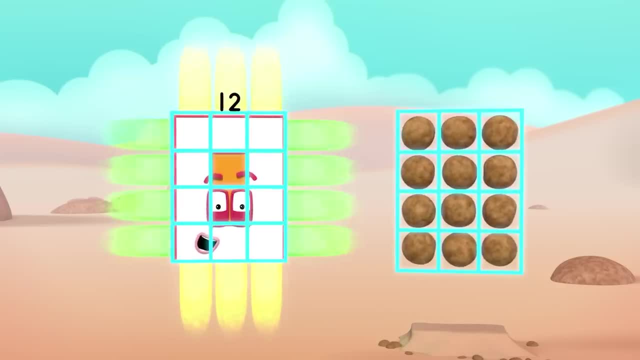 And that's called Array, Array. Hey, I'm rectangular twelve, I'm ten and two, I make arrays. that's what I do When I put my blocks in columns and rows. I make an array and my rectangle goes. 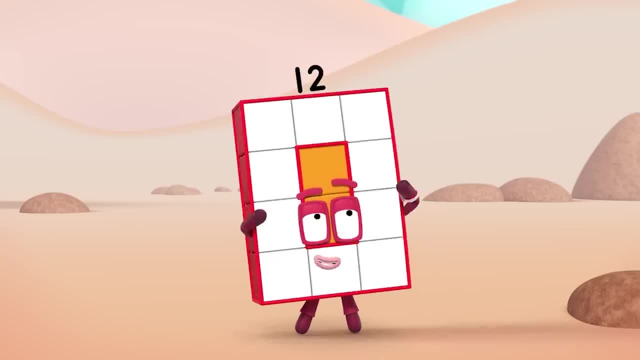 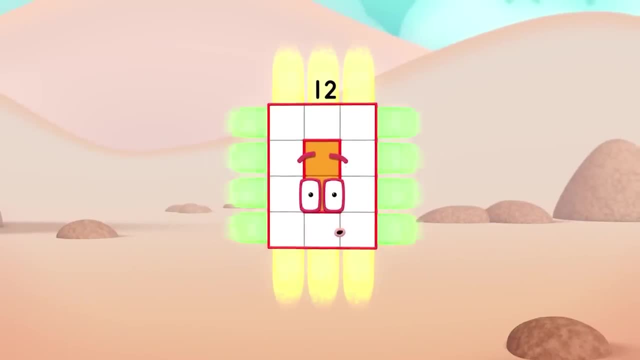 Like this, Three By four. Today's the day for an array display. I can make arrays all day. I make arrays in many ways. Stand back, let's play Arrays away. Arrays, Arrays, Arrays, Arrays, Arrays. 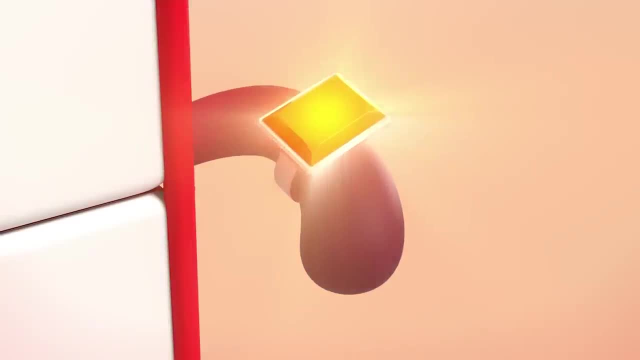 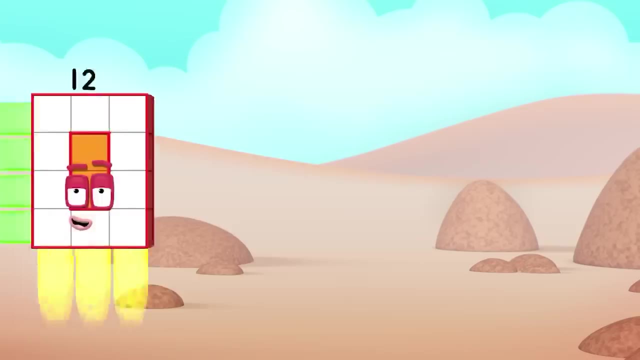 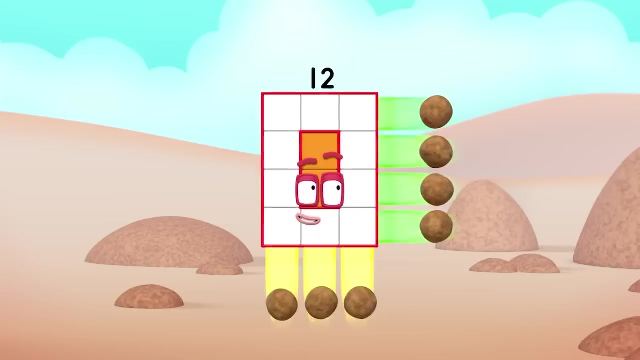 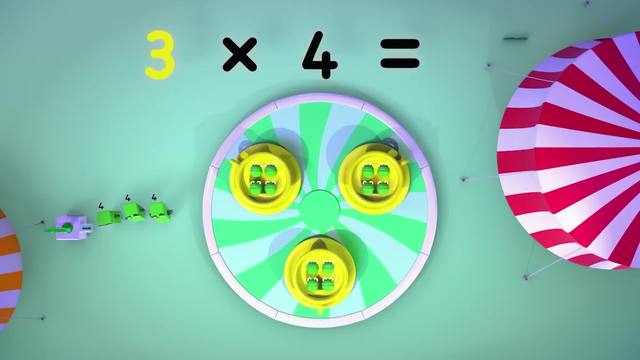 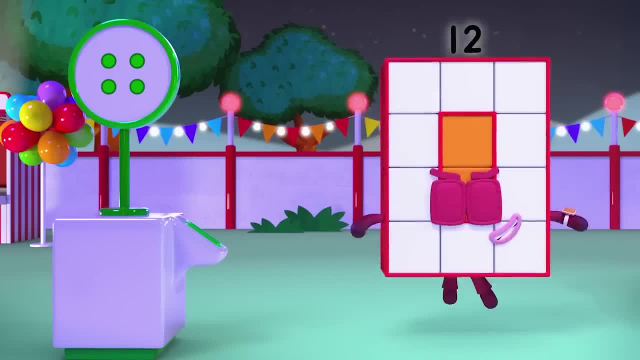 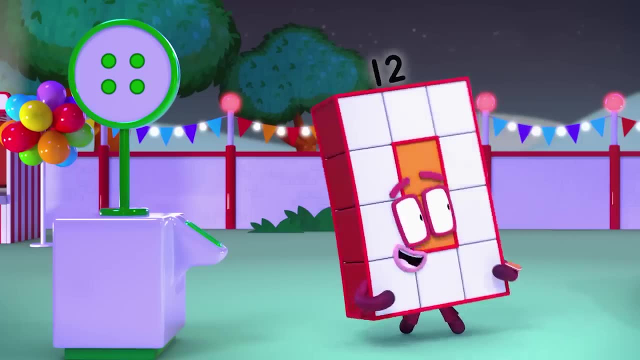 Two, Three by four, Stiff, All right. Three by four, Stiff, Three by four. There we go, One by one. It's your life, You can do it. You have that, You can die. Three lots of four, twelve number blocks and not one more. 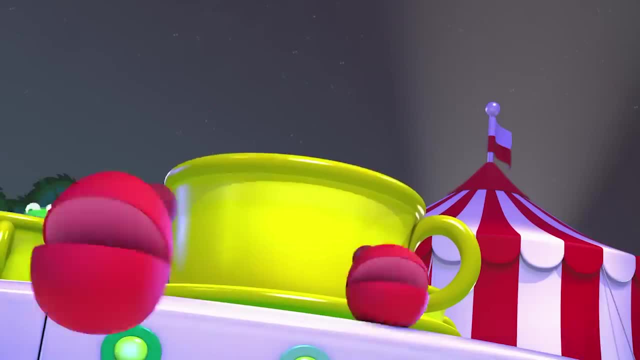 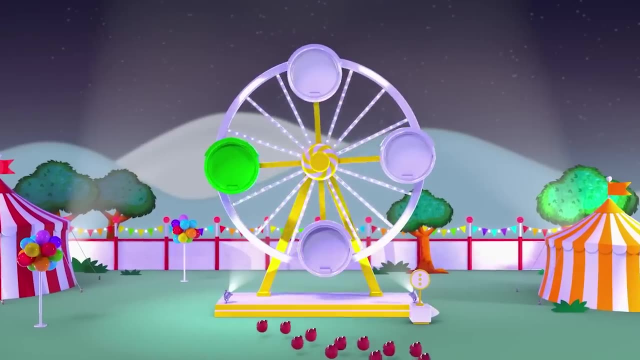 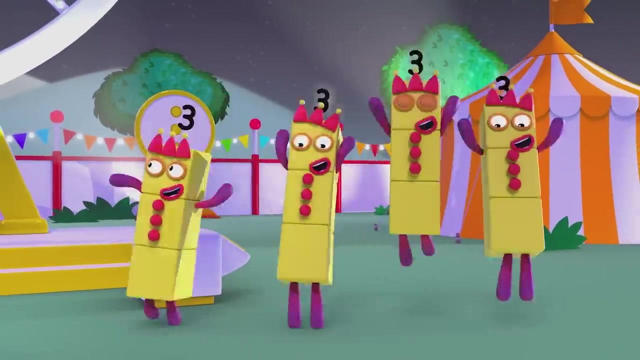 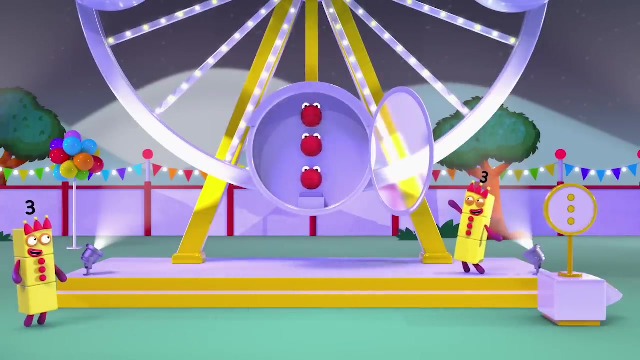 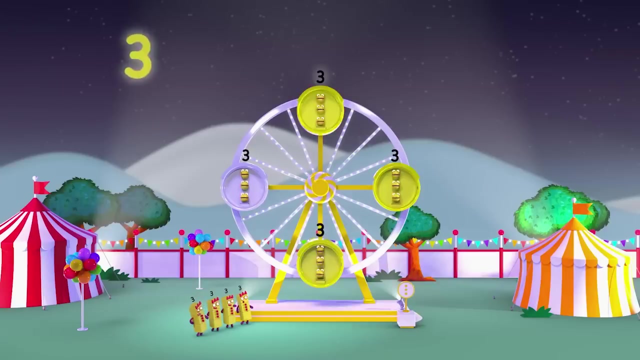 Three, That was fun. The big wheel. the big wheel Looks like three to a carriage this time: Two, Three, Three, Three, Three, Three Time for tokens. How many carriages? One, two, three, four. 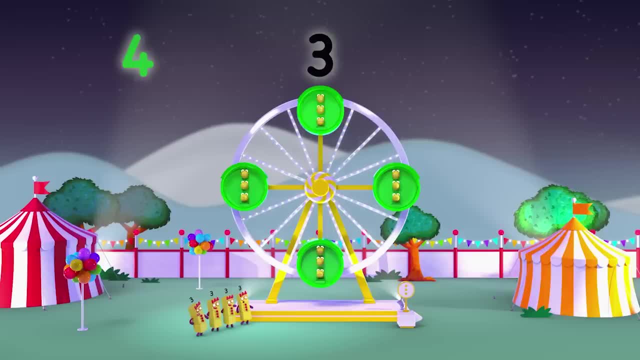 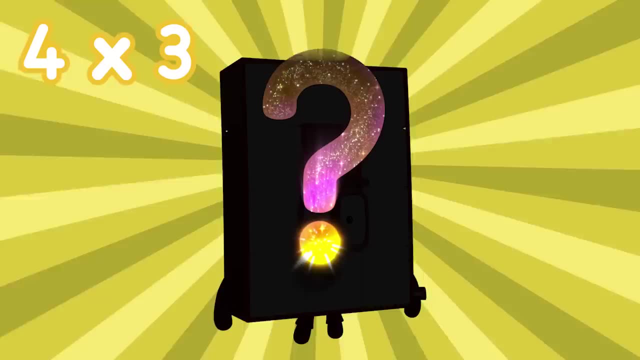 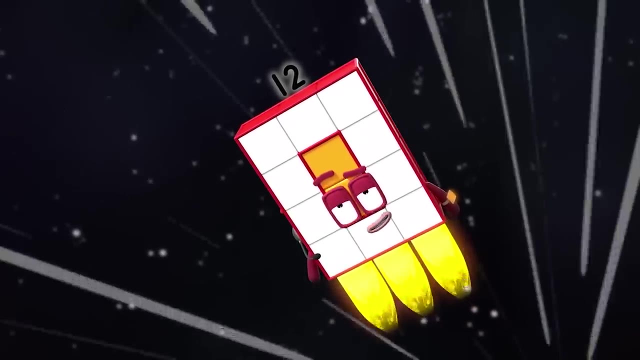 How many in each carriage? Three. So how many tokens do you need? Four times three equals Twelve. The block is no more If you match for a super rectangle like me. all teams report in Switch Two sixes standing by. 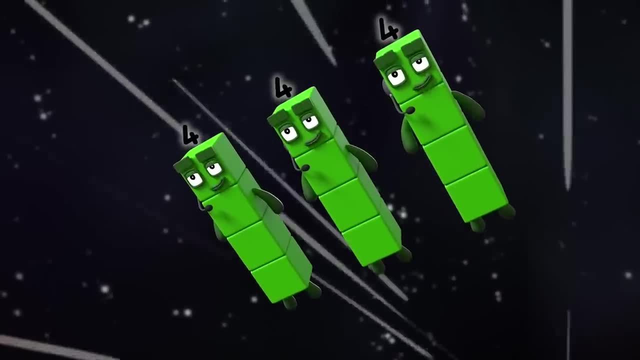 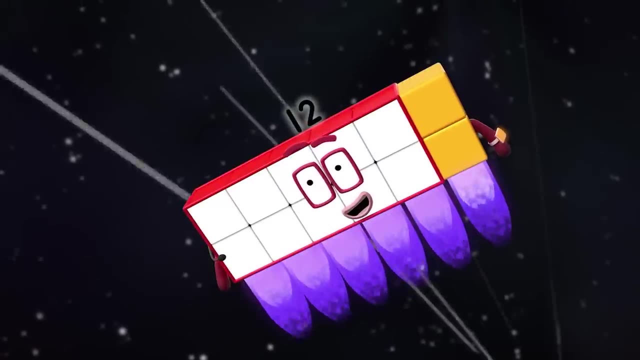 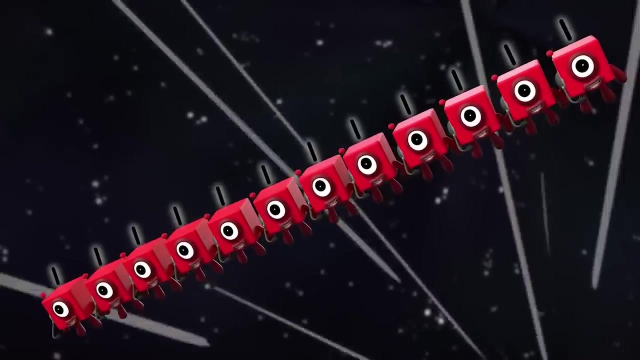 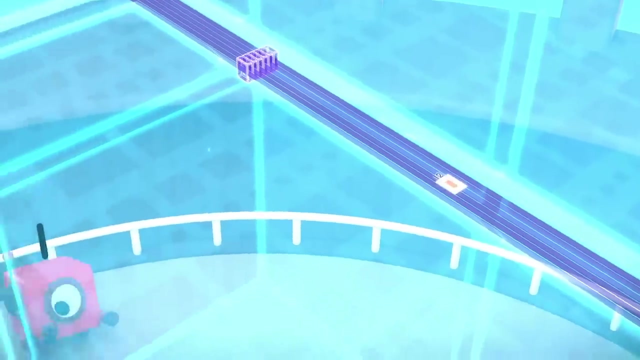 Switch Three. fours standing by Turn Four. threes standing by Switch. Six. twos standing by Switch. Twelve ones standing by Switch. I'm going in. Hold on tight. You need to turn off the force field before you can get to the battery. 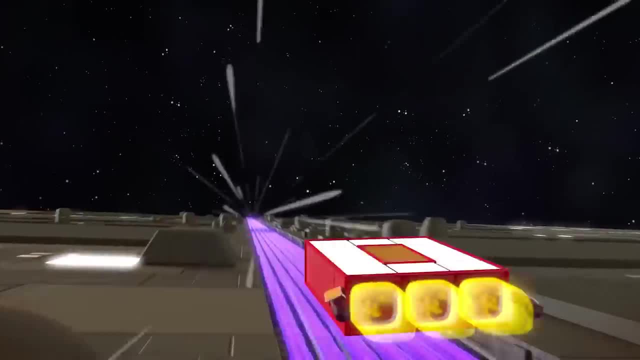 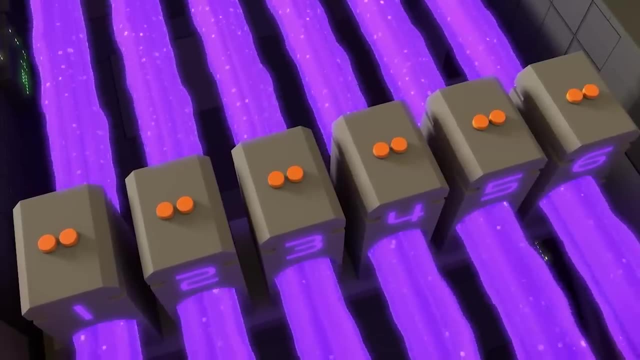 Can you see a line of towers ahead? Yes, Six of them. Each has two buttons on top. You need to press all the buttons together. Six towers, two buttons each. Array display. This calls for switch, Switch, Switch, Switch. 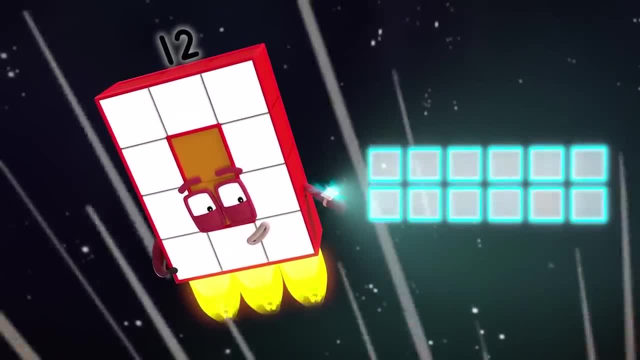 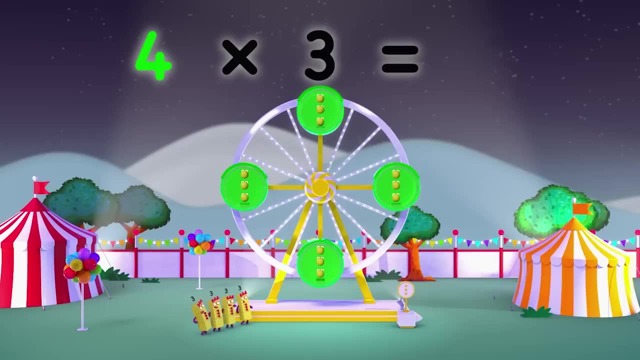 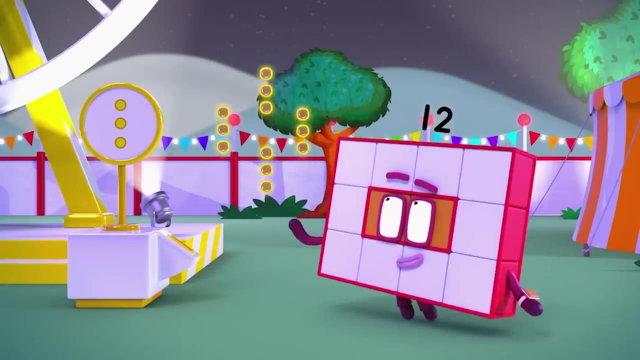 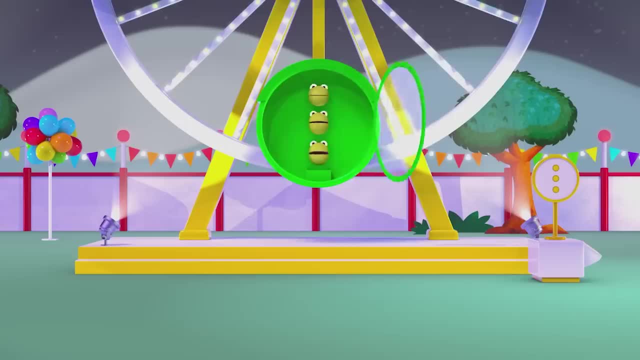 One, two, one, two, three and go Perfect, save your games. That was perfect. So this is a cult. No bueno, Ah, my Islam 와서 where you're going. thanks, Here you go, Myagen. 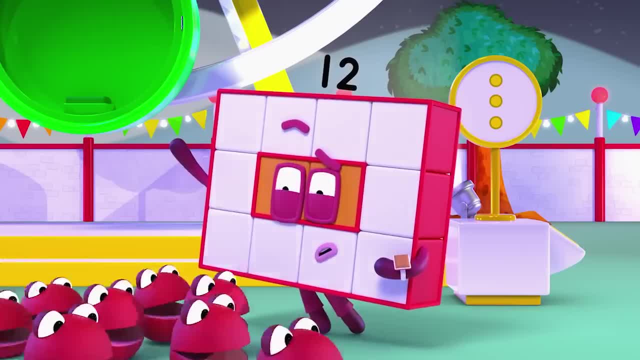 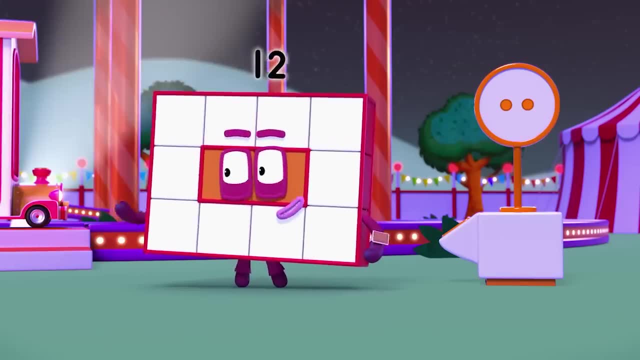 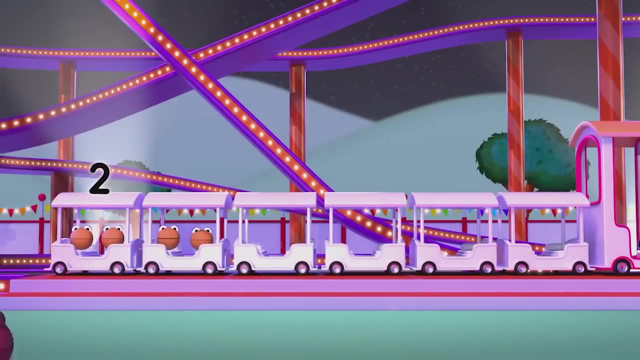 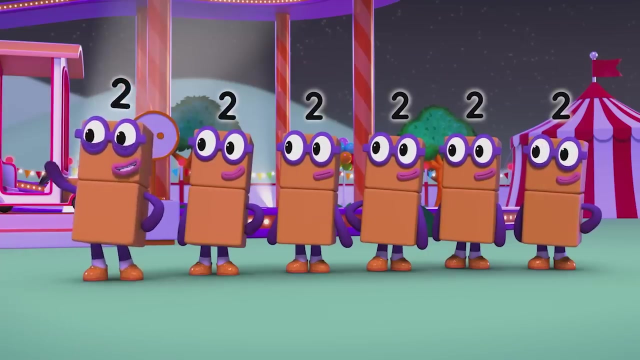 The runaway train. The runaway train In pairs. please Switch All aboard. Two, two, two, Two, two, two. Now how many carriages are there? One, two, three, four, five, six, seven, eight. 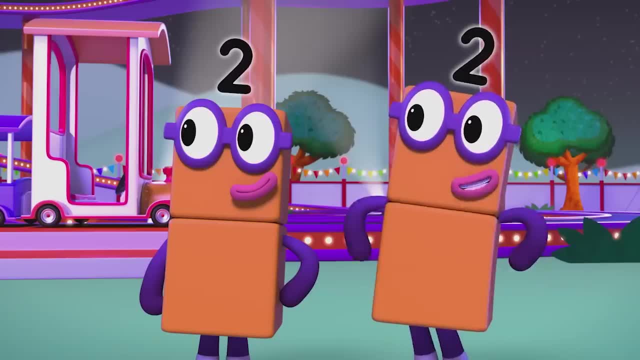 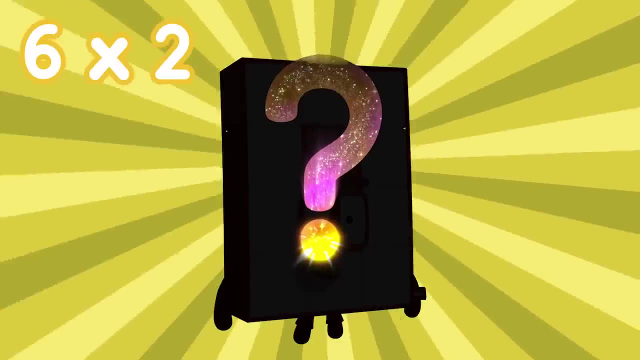 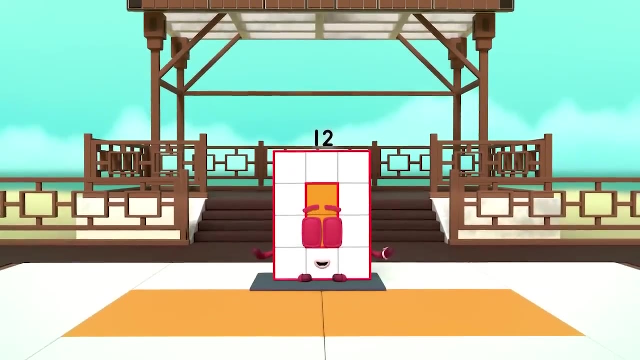 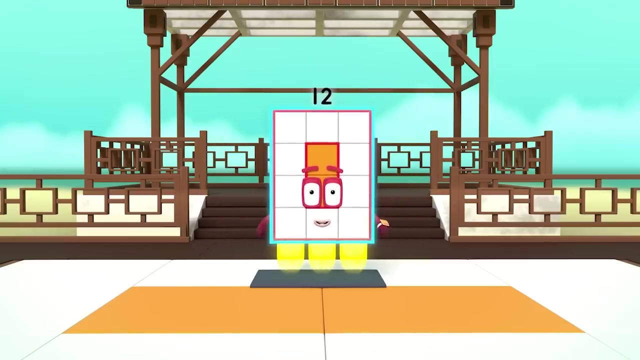 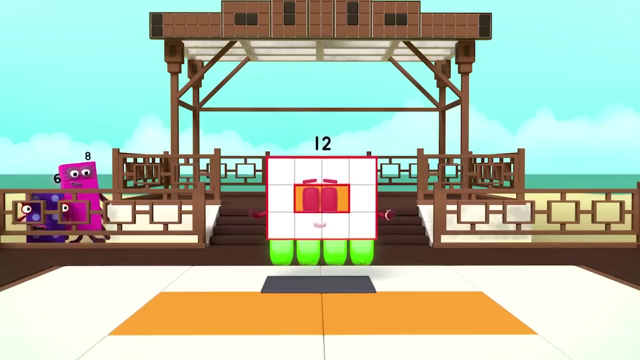 Four, five, six, And how many in each carriage? Two, Six times two equals Twelve. I am twelve, I am three by four, I am a rectangle. I am also four by three And I am a super rectangle. 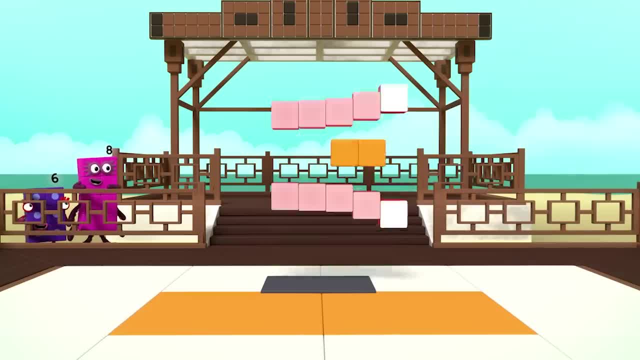 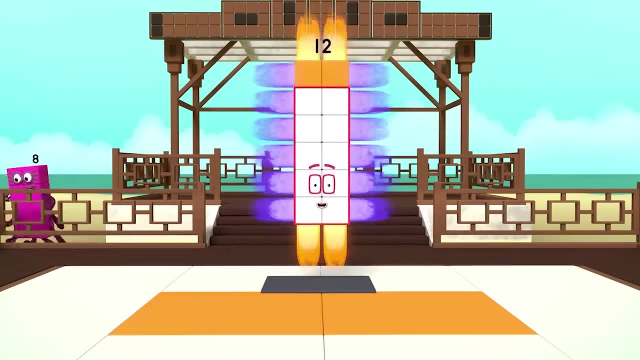 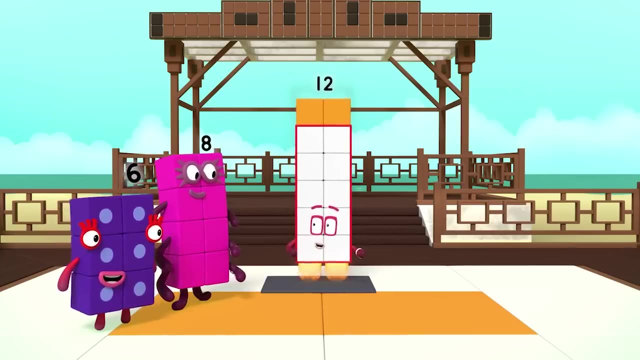 I can take many forms. Switch: I am six by two. Turn. I am two by six. I am a rectangle. Welcome, my friends. Would you like to master the way of the rectangle? First you need to stand, so your front makes a rectangle shape. 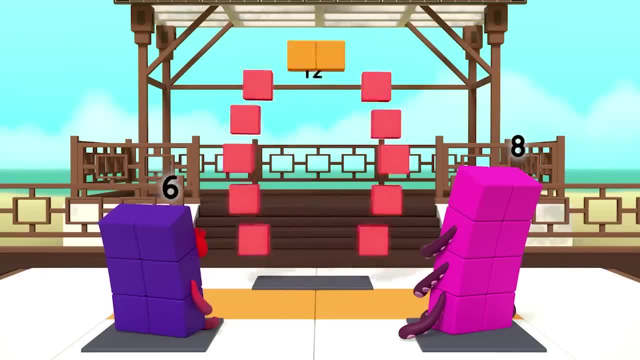 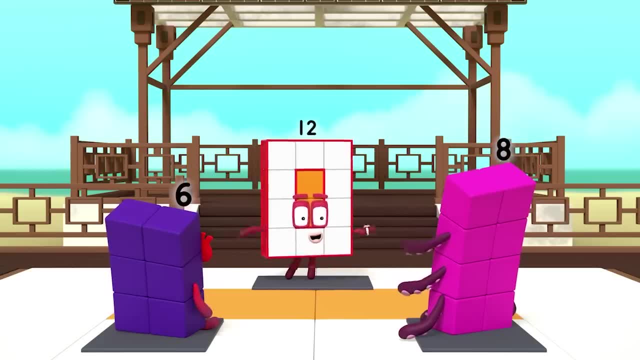 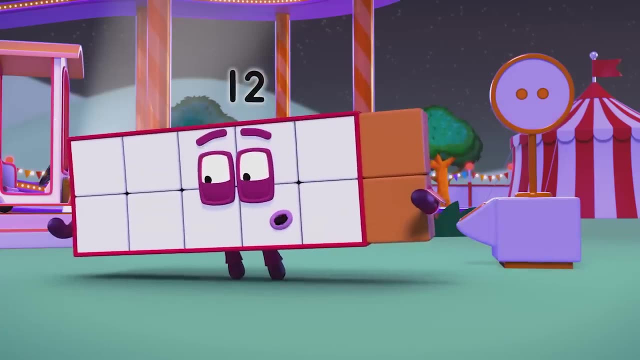 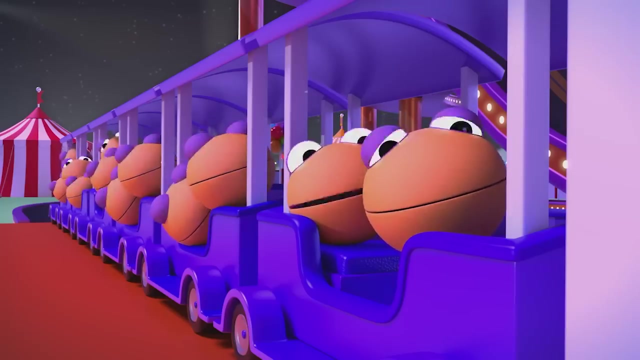 Watch and tell me when I'm making a rectangle. No, No, Yes, Well done. Now look at your own fronts. Twelve, So you need twelve more. Oh, I'm all out of tokens. Oh, Oh, Oh. 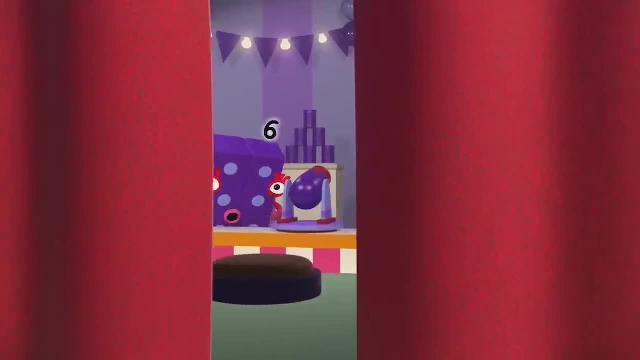 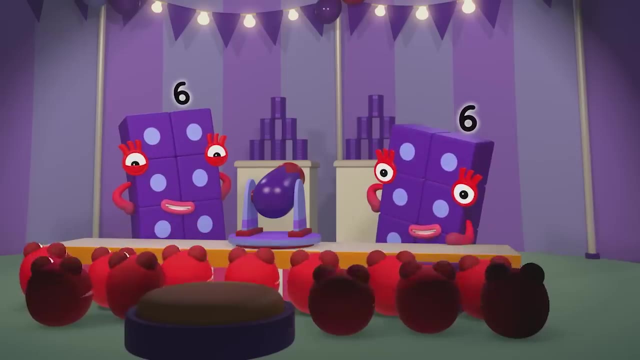 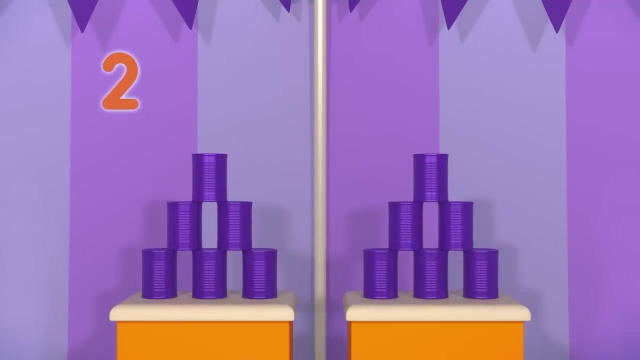 Oh Huh, Roll up, Roll up And have some fun. There's lots of tokens to be won. Ooooh, We need twelve tokens. You'll win one for each can that falls, And there's One two. 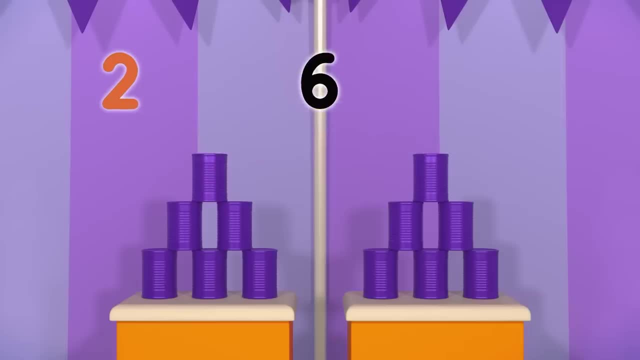 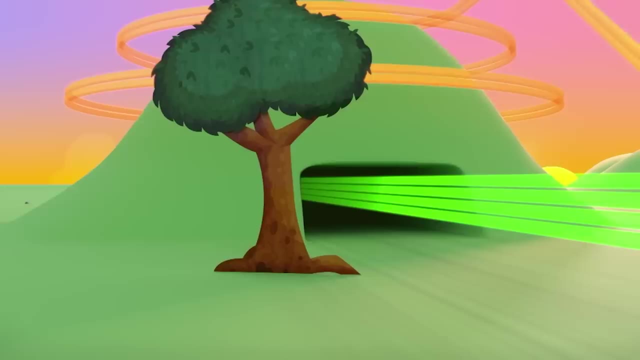 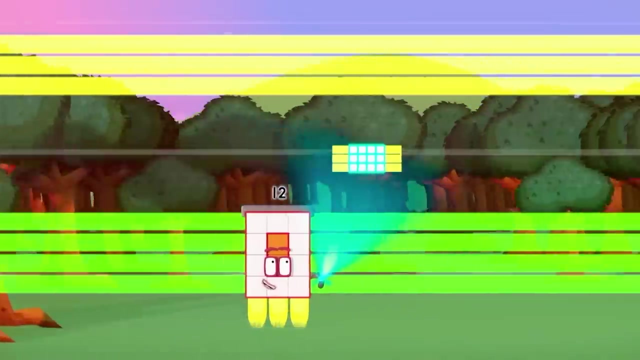 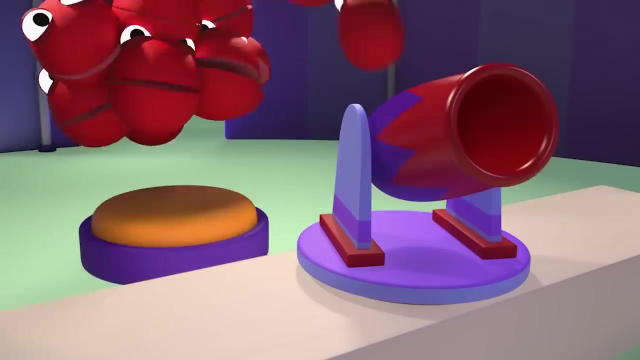 Two stacks, One, two, three, four, five, six equals 12, 8 rays. I can't make an 8 tall rectangle, but I can write 3 rays, 4 by 3, 12, Hooray, Hooray. 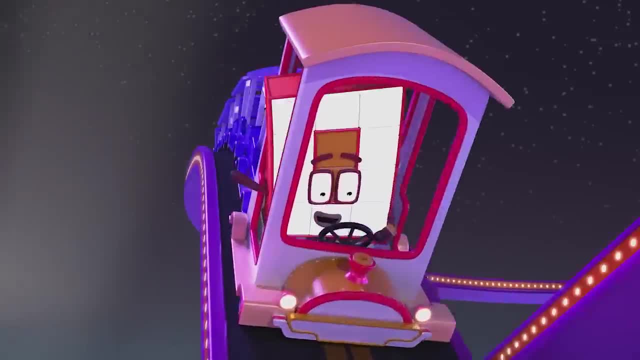 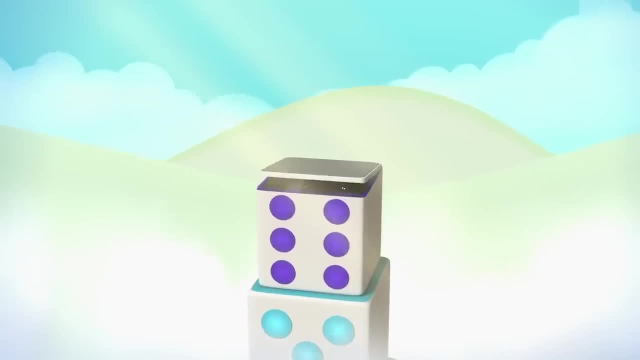 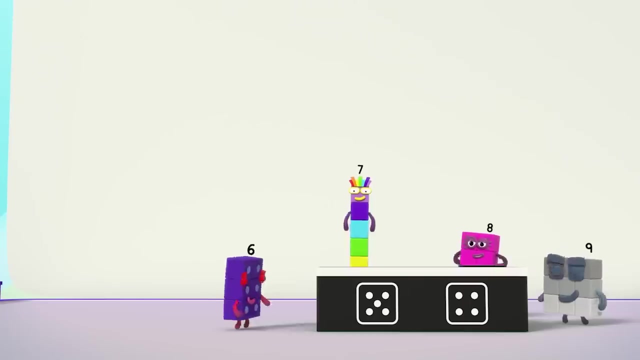 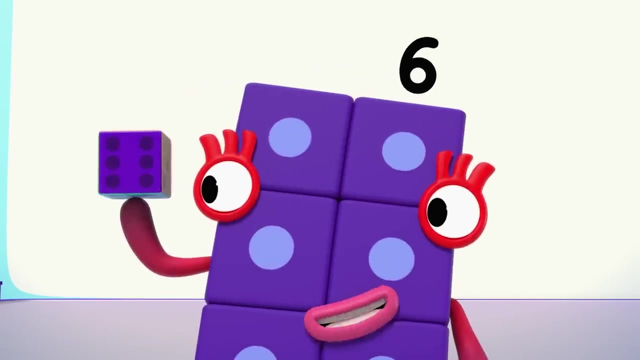 Here we go. 6 lots of 2, 12 number lots. Choo-choo-choo-choo. Thank you for coming to play my big new game. I'll roll the dice to start my friends, This game is called How Many Tens? 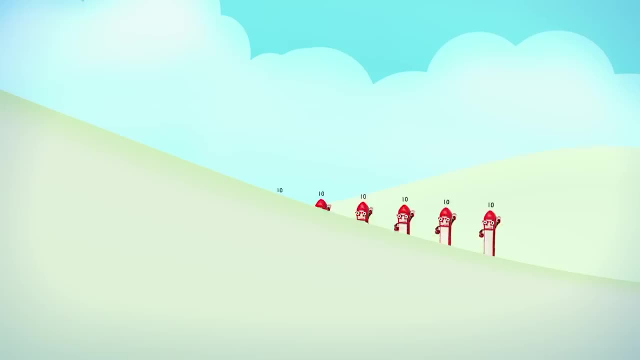 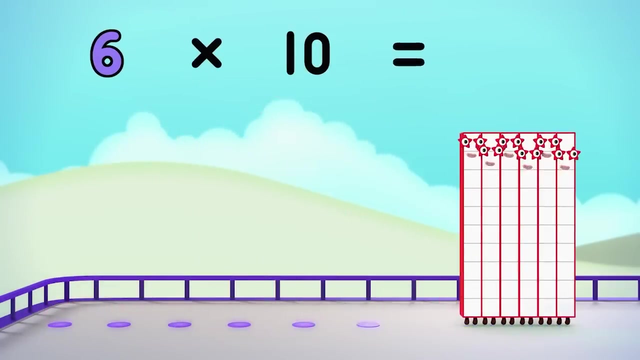 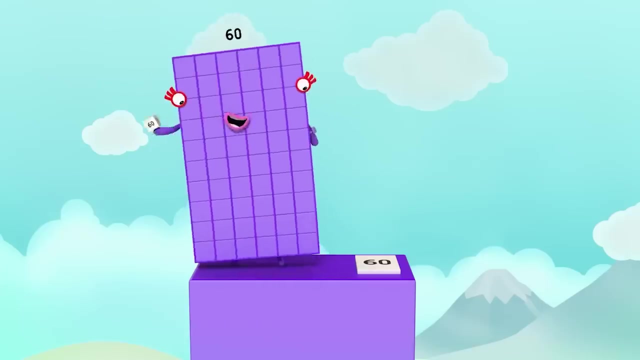 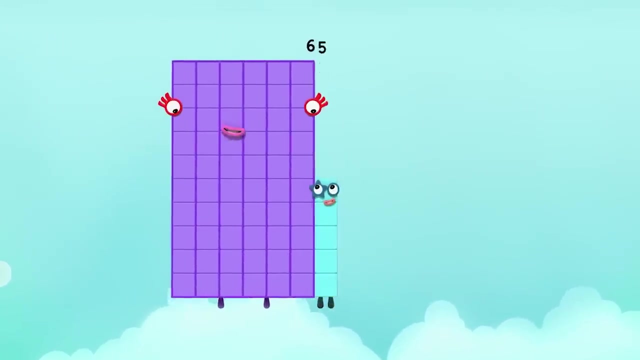 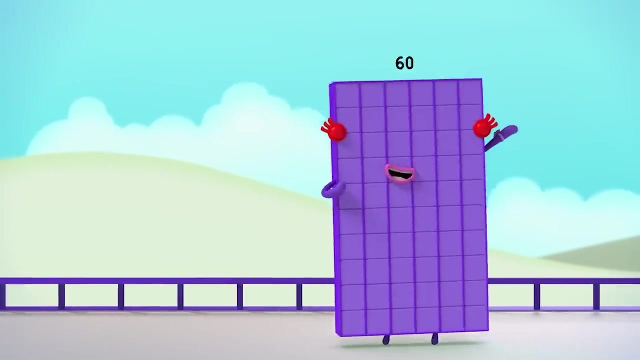 6, 6 times 10 equals 60: 60. Racing through the sky, This high roller's gonna fly. 61, 62, 63, 64, 65, 66, 67, 68, 69, 60, 70. I am 60 here to play. 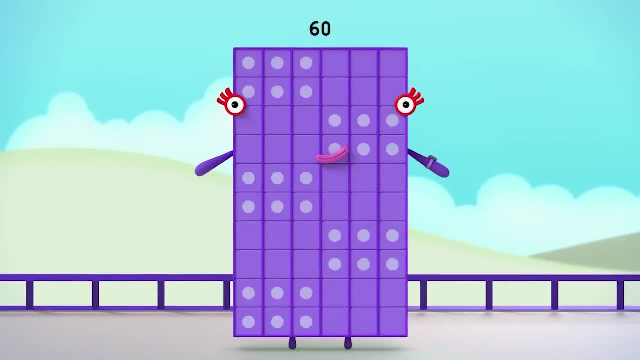 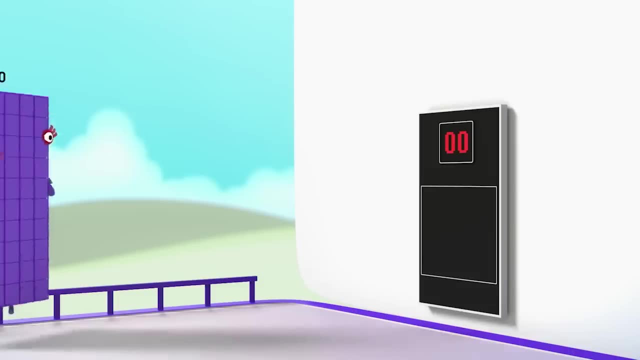 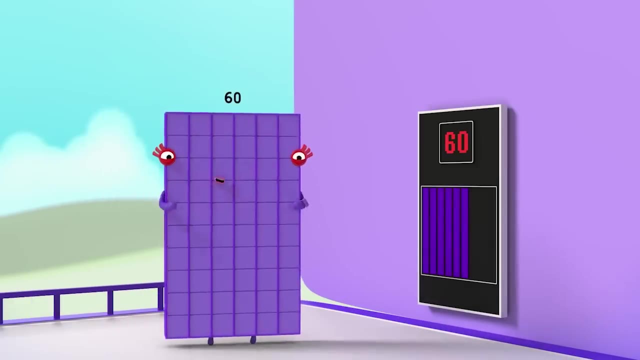 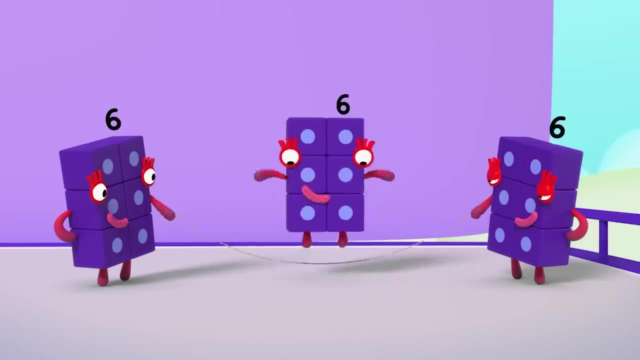 With 60 spots. Hip, hip, hooray, Wow, 60, 60, 6, lots of 10 is a new high score. I'm 6 tens or 10 sixes. Game on. Yeah, Hee, hee, Hoorah, Hoorah. 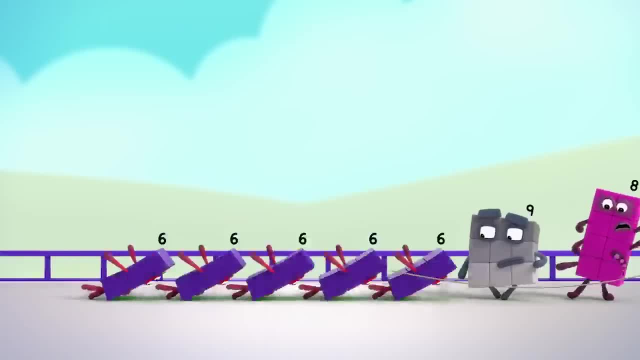 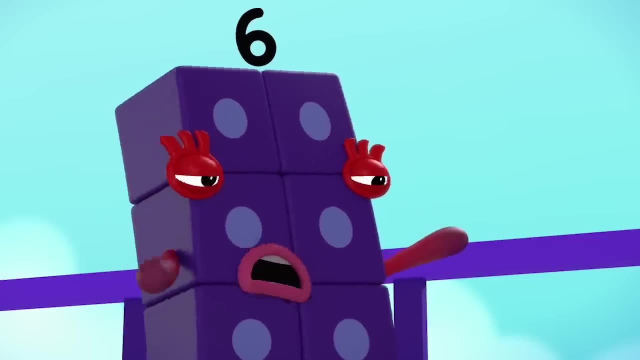 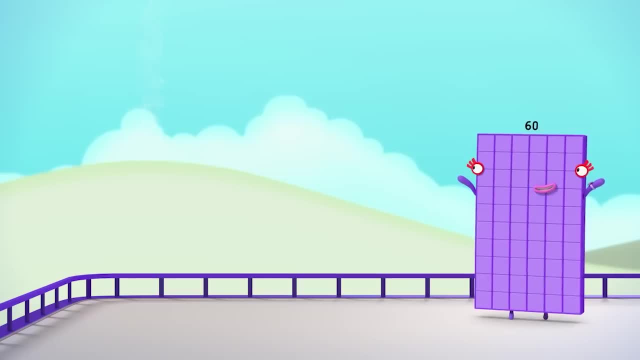 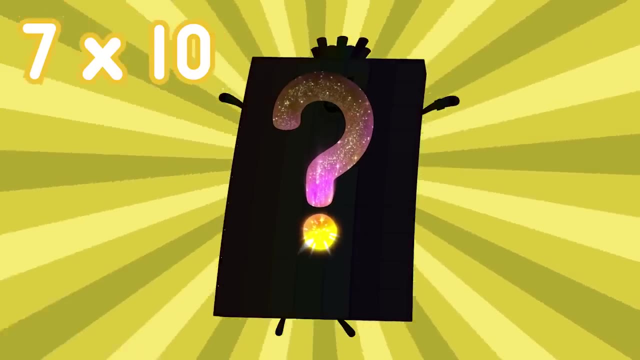 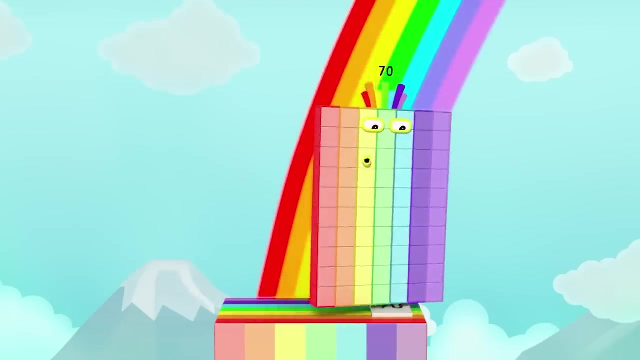 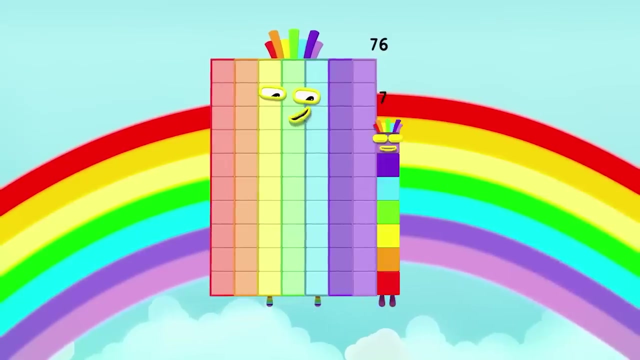 This calls for another 10!. 7 times 10 equals… 70!. Hooray, 7 times 10 equals… 70! 70! 70! 70. we're going over the rainbow. 71, 72, 73, 74, 75, 76, 77, 78, 79, 80. 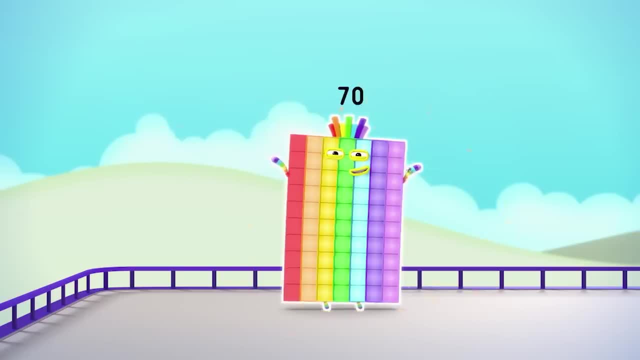 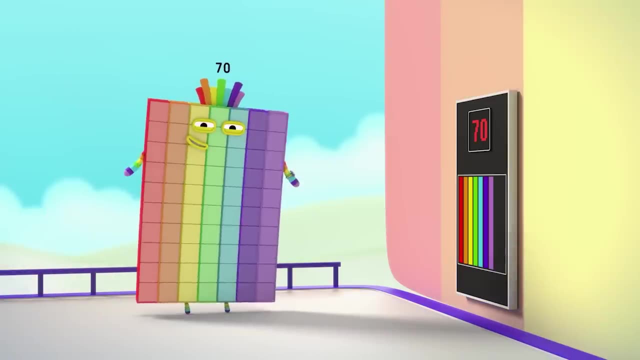 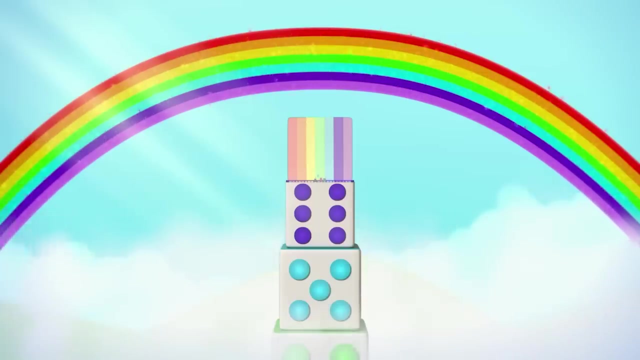 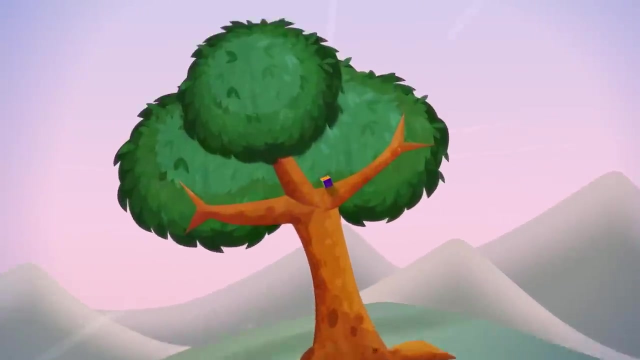 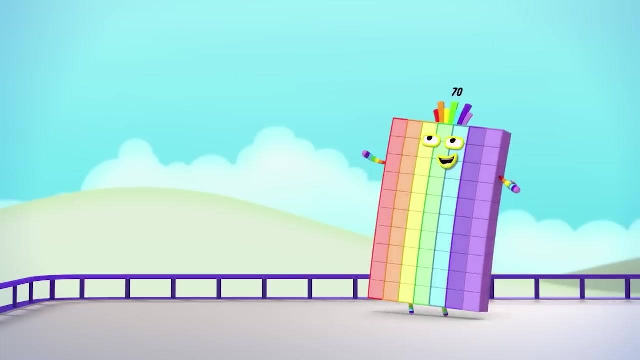 70.. i am 70.. new lucky numbers, as luck would have it, i'm seven tens, so i'm also ten sevens. the rainbow connection, i see it. it's way over there, but how can we get it back again? luck is in the air tonight. here comes another ten. 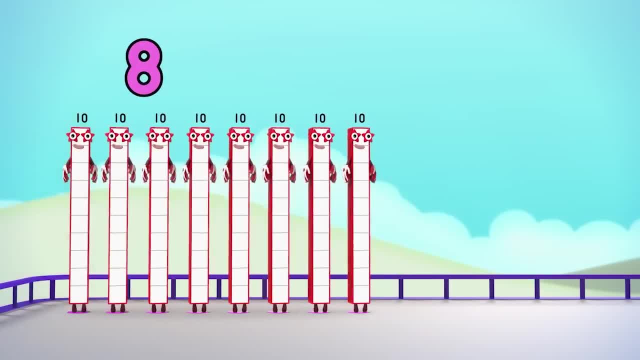 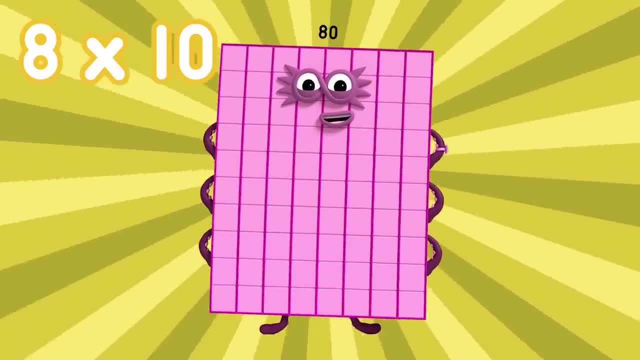 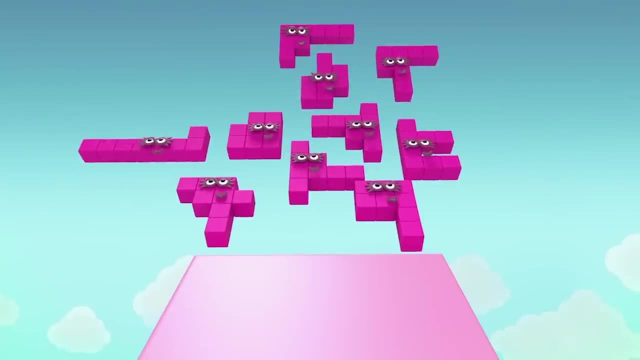 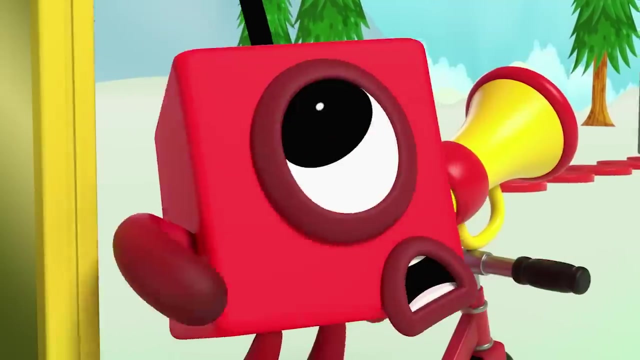 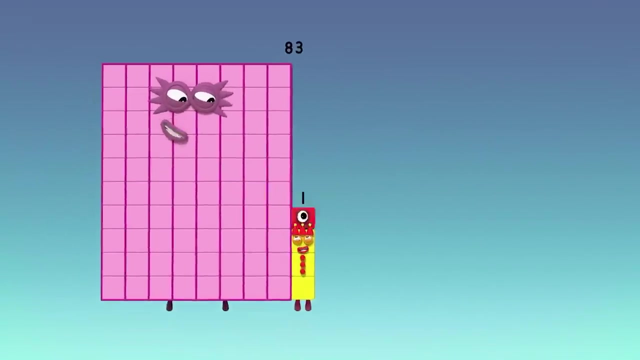 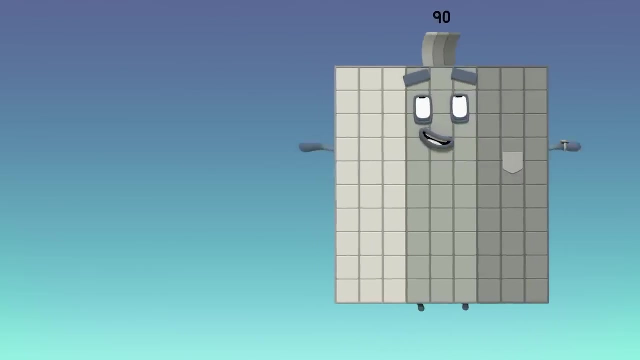 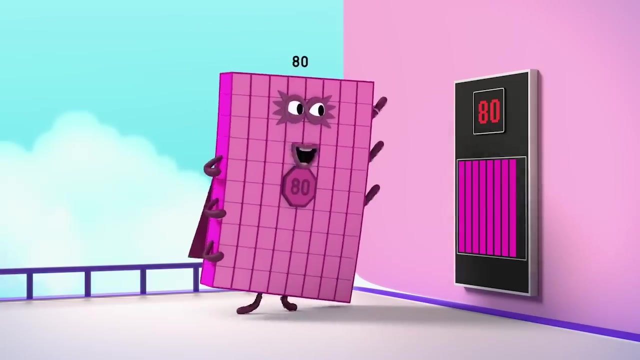 eight times ten equals 80.. i don't like the look of those clouds. there's no time to stop. octoblocks. assemble dino block, raw up, up and away. 81, 82, 83, 84, 85, 86, 87, 88, 89, 90.. 80.. i am 80.. super octoblock: to the rescue. 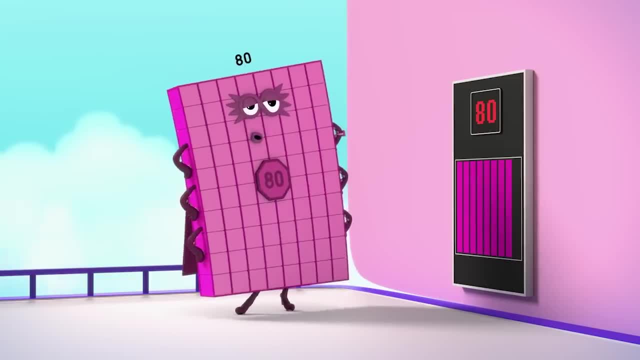 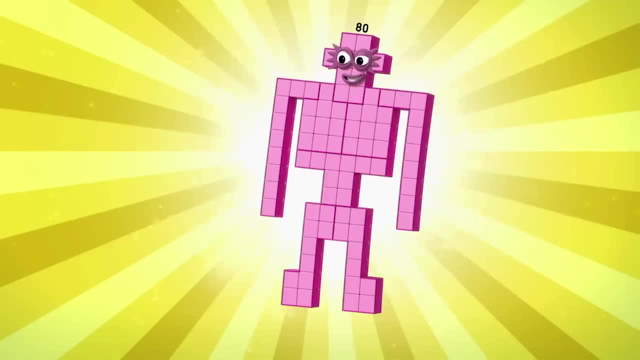 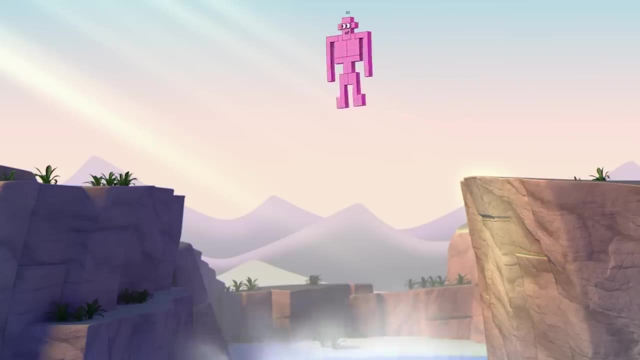 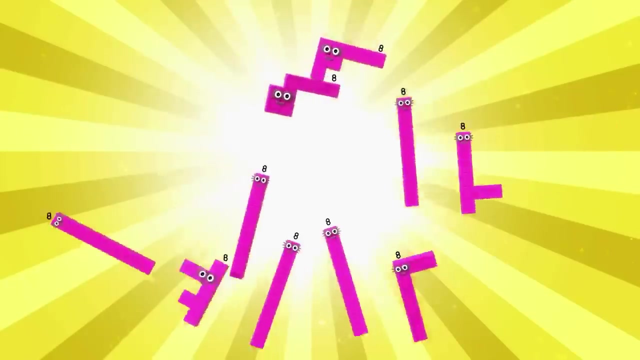 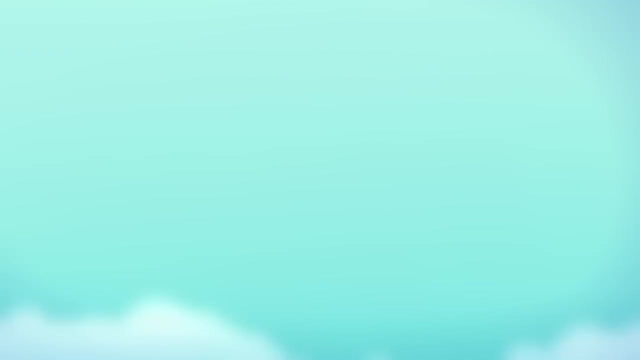 secretly, i'm eight tens, but this is a job for ten. eights, octoblocks. assemble the octoblock forward, dinoctoblock smash. 80's the biggest hero of all. oh, there's always someone bigger look. 80's the biggest hero of all. oh, there's always someone bigger look.